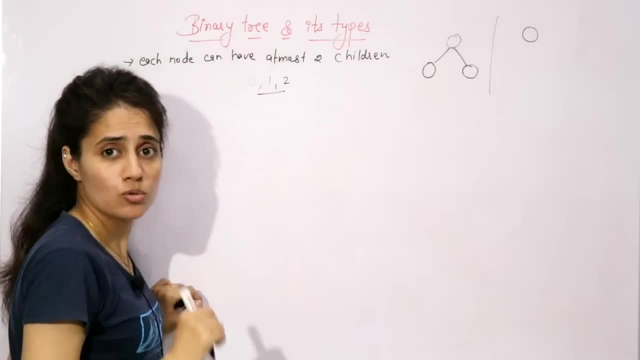 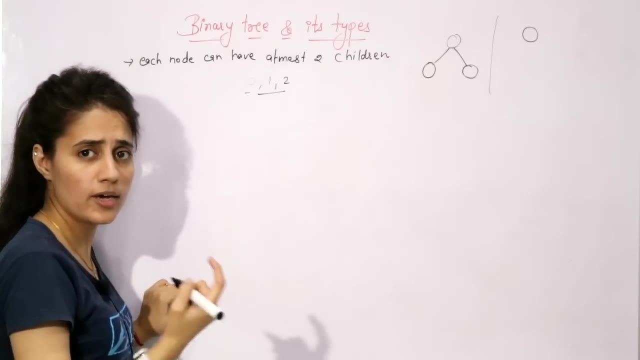 Now, is this a binary tree? Yes, This is also a binary tree. This is having only one node, That is, root node. Having no children. That is possible. We can have zero child. A node can have zero child, right? So this? 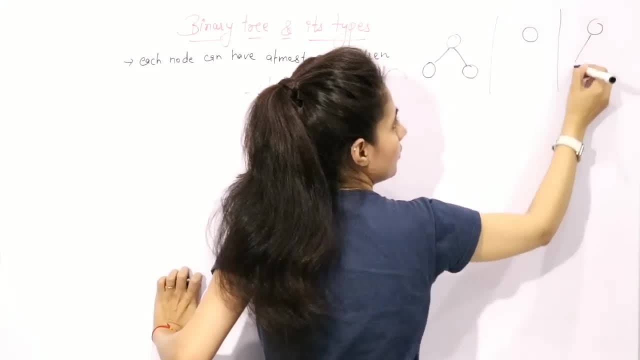 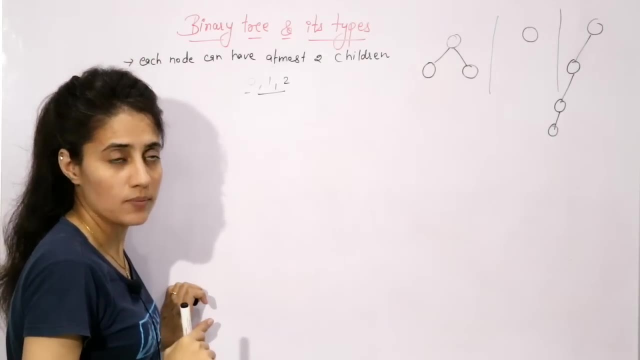 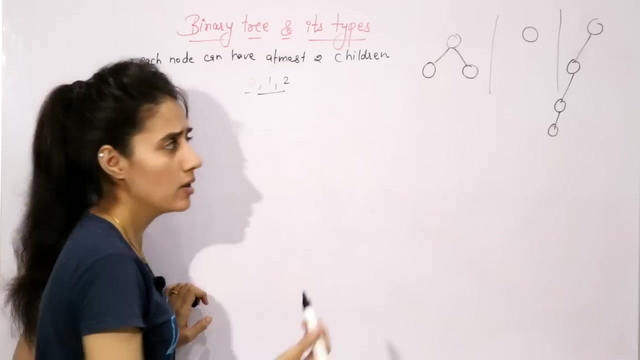 is also a binary tree. Now see, what about this one? Is this a binary tree? Yes, This is also a binary tree. See, here each node is having. this node is having one child, one child and one child. This is having zero child. That is also possible. Now see. 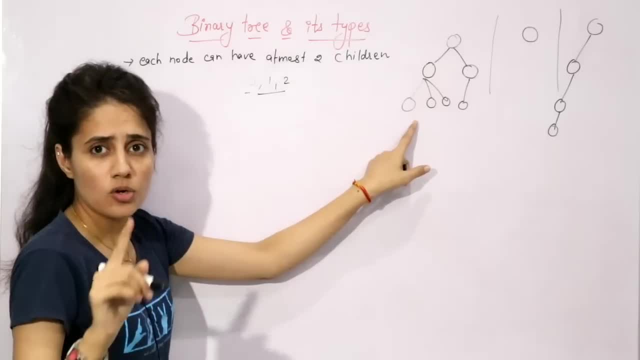 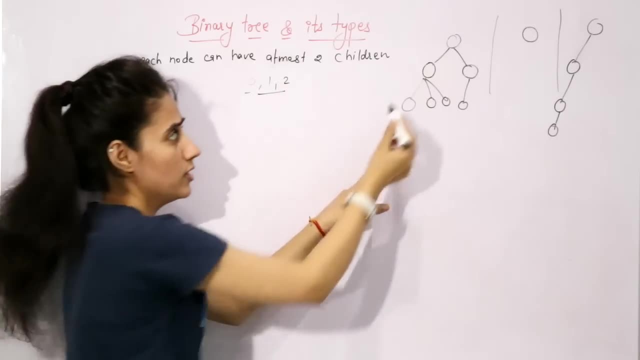 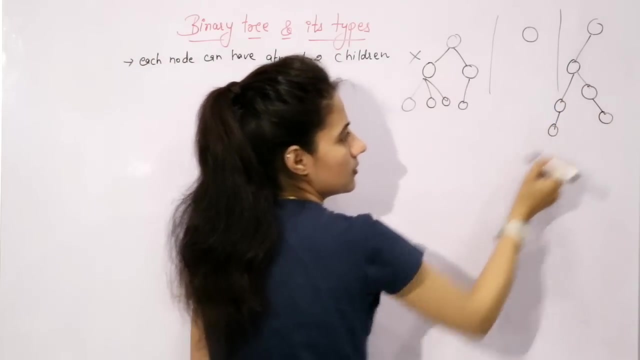 Is this a binary tree? This is not a binary tree because, see here, in this case, this node is having three children. That is not possible. We can have, at most, two children. So this is not a binary tree, right? All these are binary trees. This is also a binary tree, right Now, if I draw something like: 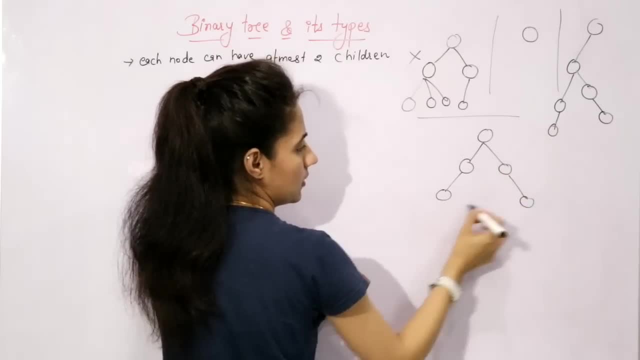 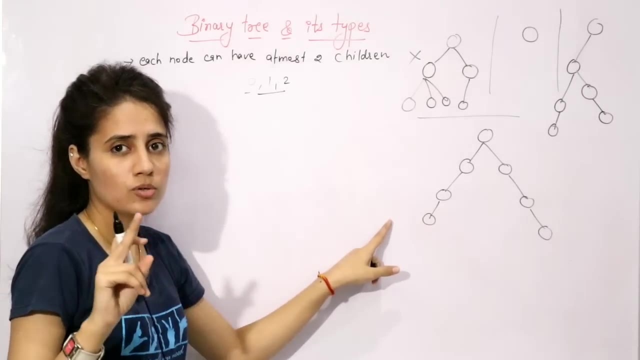 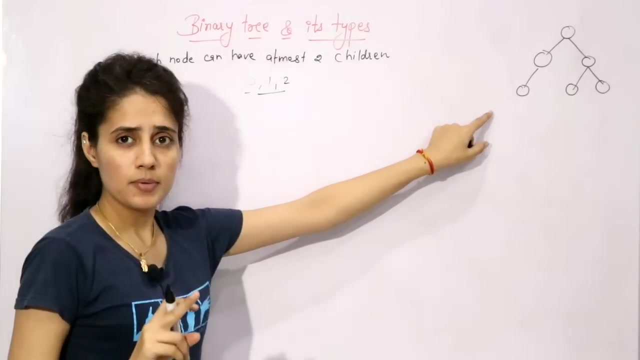 this, This, this, this and this. This is also a binary tree. The only condition is what Each node must have at most two children. If this condition satisfies, then that is a binary tree. Now, how we are going to represent this binary tree in memory, that thing we have already discussed in. 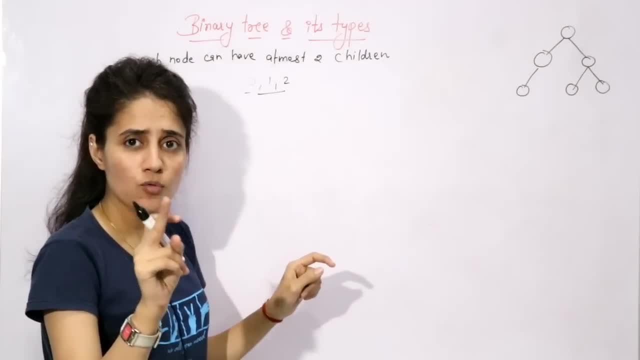 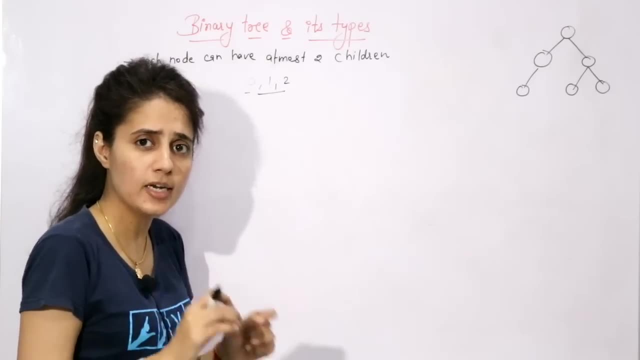 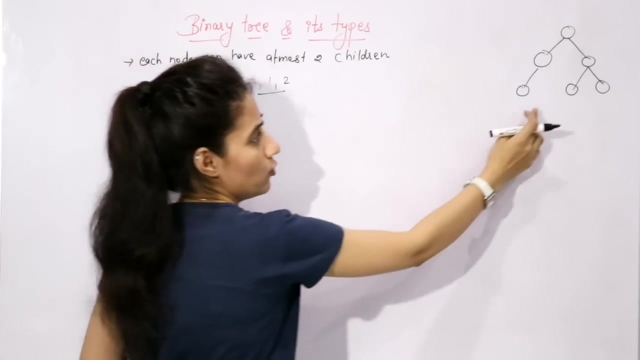 the previous video, See here. this is the node. Each node is having what Information, plus may or may contain links. That is not compulsory that each node should contain link to another node. Maybe if node does not have any child, then it will not contain any link, right? So how you are? 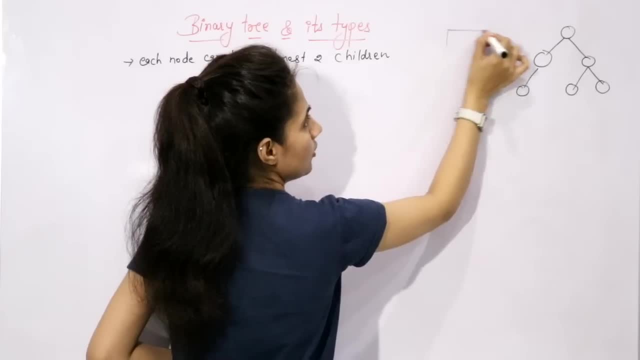 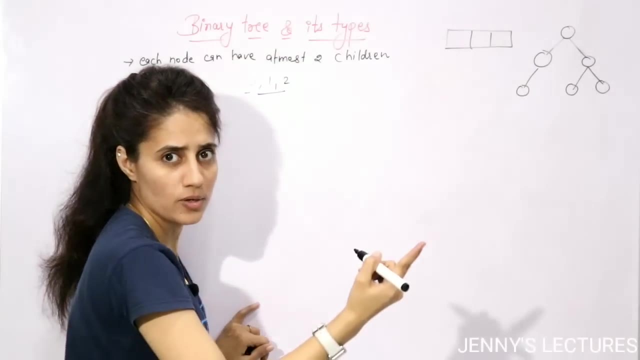 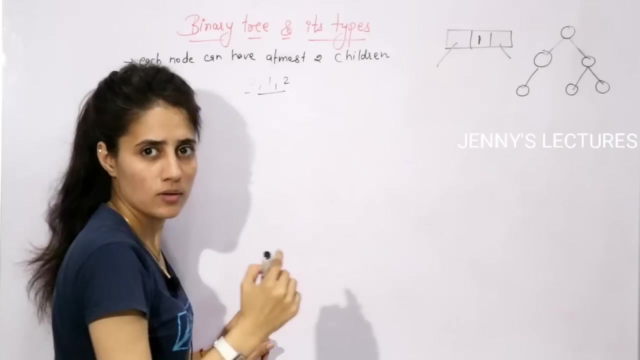 going to represent this binary tree. see, this is a node. first node is something like this: three parts would be there: this is what left child, this is what right child. you can say: so here we have the data part. you can say: here i am storing one, this is what left, this is what link to the right child. so here we have one node, this 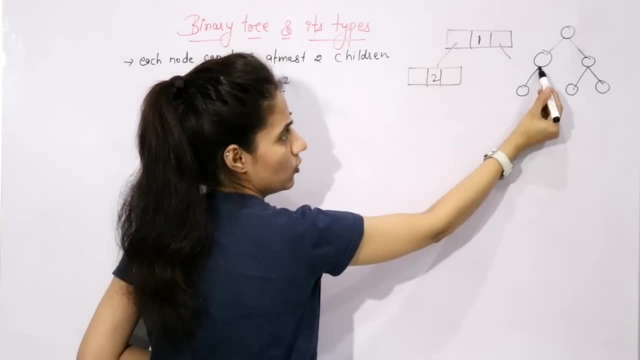 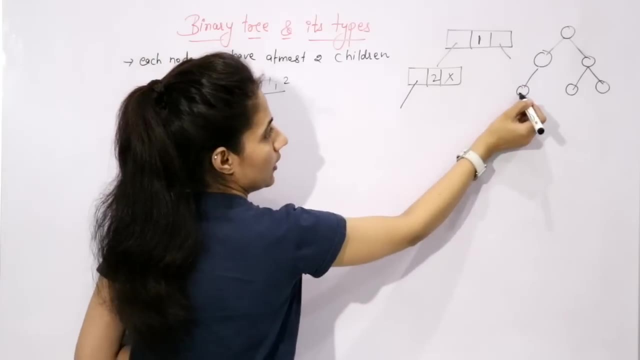 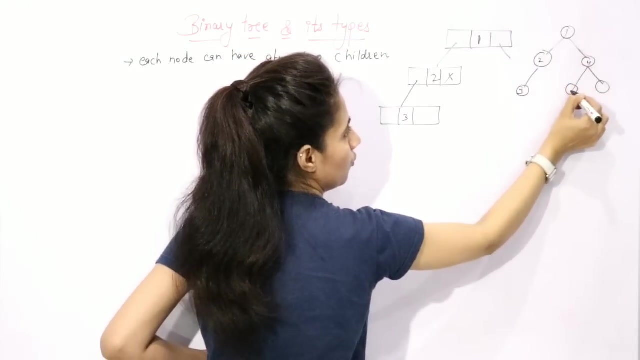 node is suppose having data two. now see, this node is having only left child, so this is having only this link. this link is null, right. so now here, this is also suppose containing three value: one, two and three. here i have four, five and six, because these node are having some information. 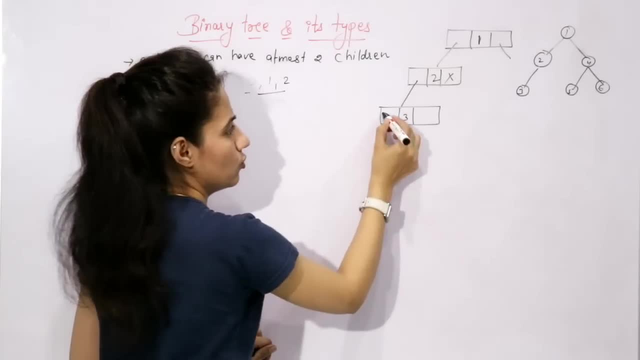 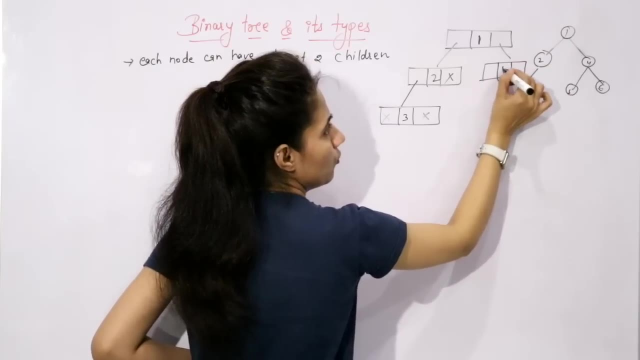 stored there. three is not having any child node, so there is no this link and this link would be null. this is how we are going to represent this one here in this side we have four. four is having both left and right child, so this is left and this would be right. 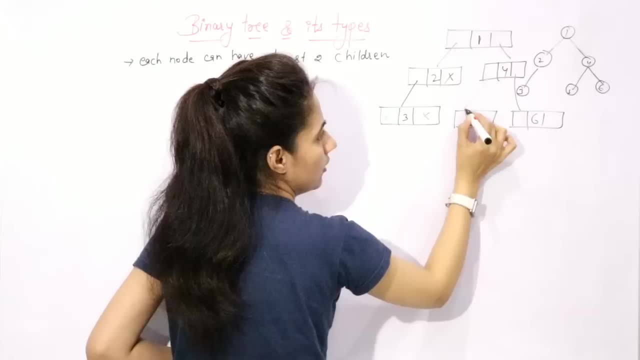 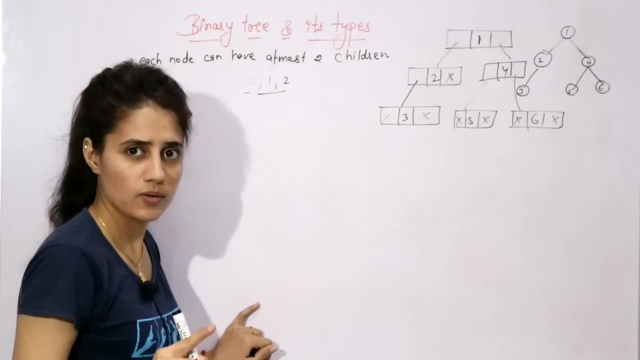 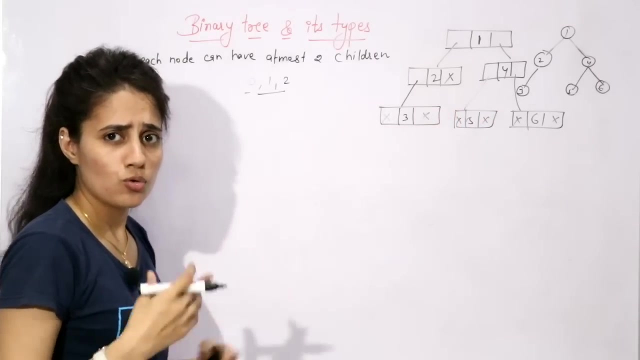 right, here we can have 5 and here we have 5 and 6. both 5 and 6 are having no children, so the links would be null, right? this is how we are going to represent the tree. actually, this is just a logical representation of a tree. how we are going to store the tree in memory. we are going to dynamically. 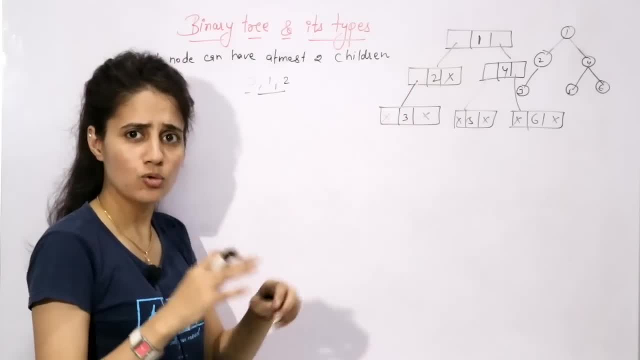 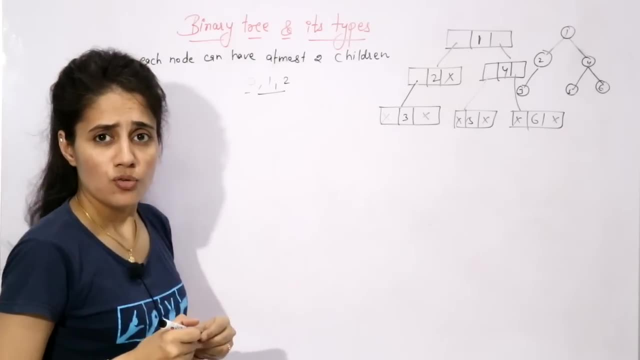 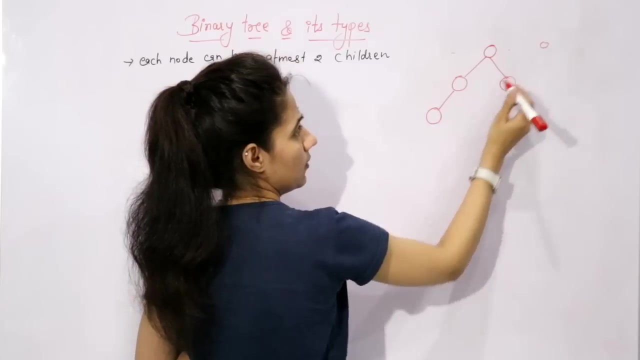 create these nodes. we are going to set these links, that thing also. we will discuss the implementation of binary tree right now. next thing is: see now some properties of binary tree. see, we have discussed what is a level in the previous video. this is node. this is what level 0. this is what level 1. this is. 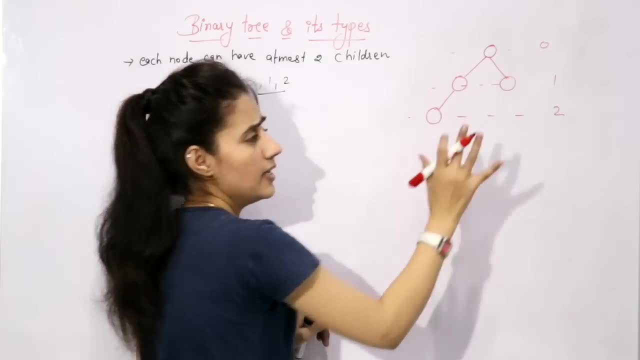 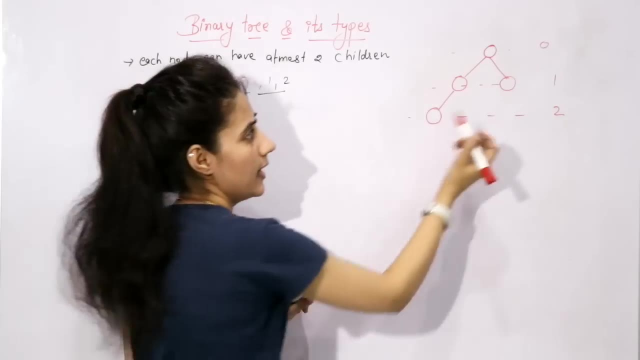 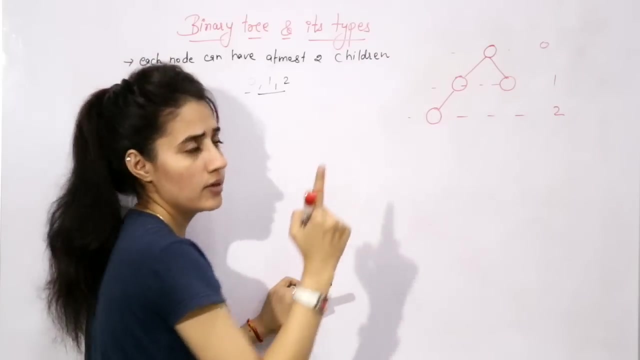 what level 2 now at any level. see, at suppose I am taking at level 1 how many maximum nodes can be possible. see: at level 1 only two nodes can be possible maximum nodes. here. we cannot have three nodes because at most two children can be there. now at level 0 the maximum node possible is: 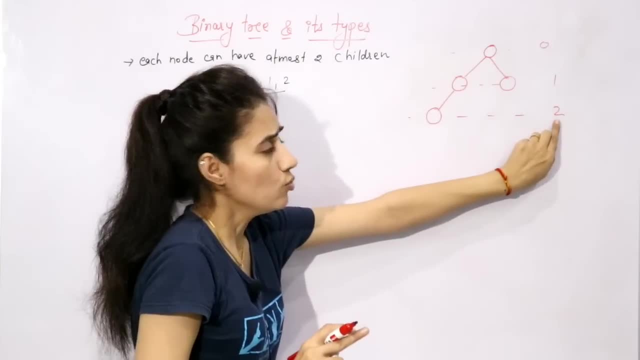 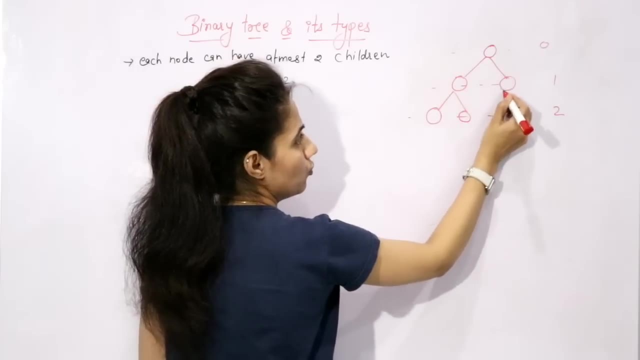 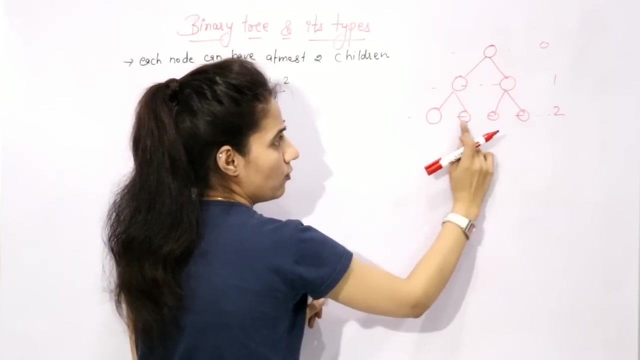 only one right. at level 2, the maximum node possible are: see the maximum node. maximum node can be here I have to. here also I have two and two children of this node. so this is what level 2. at level 2 we can have four children maximum. we cannot have five, six or something like this right, this thing. 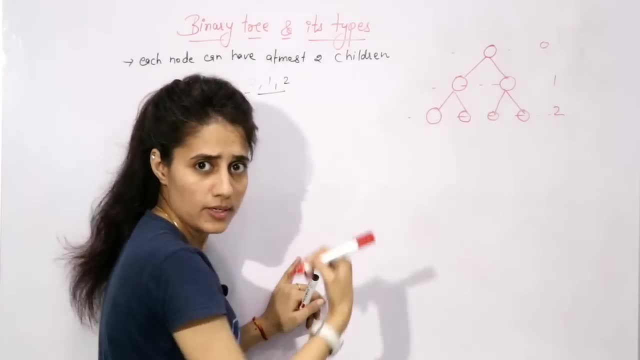 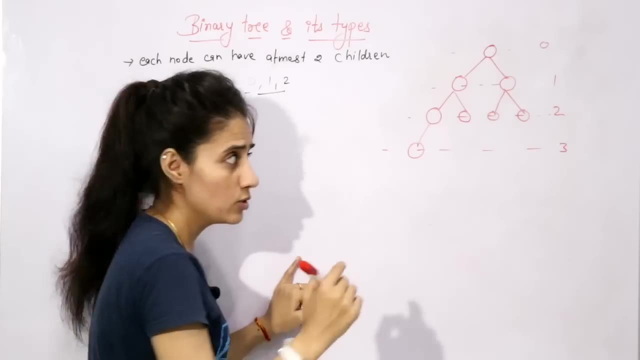 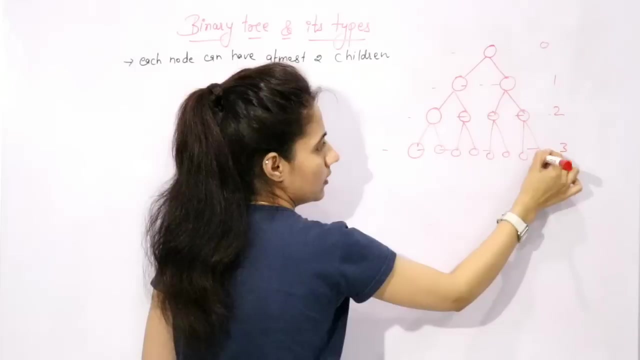 is getting my point now suppose I am increasing one level at this level. at third level, the maximum number of children possible are. maximum means each of this node is having maximum children, and maximum children can be two only. it means one, two, three, four, five, six, seven. 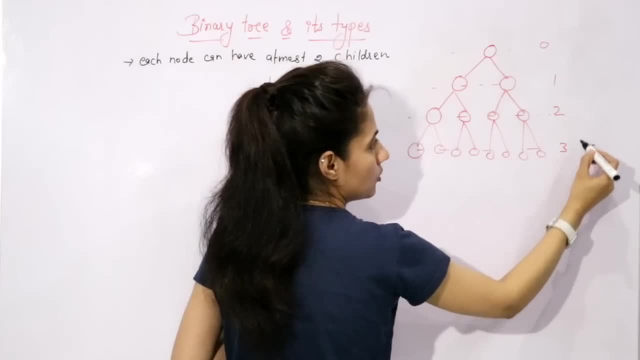 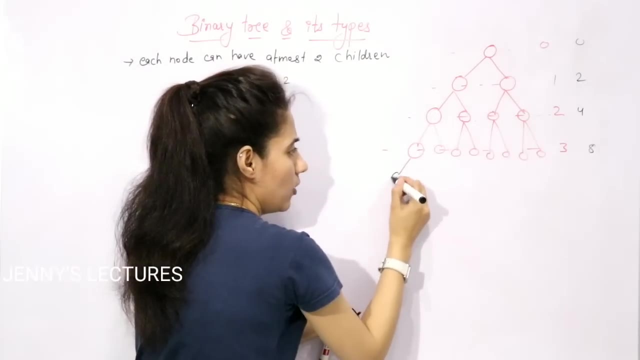 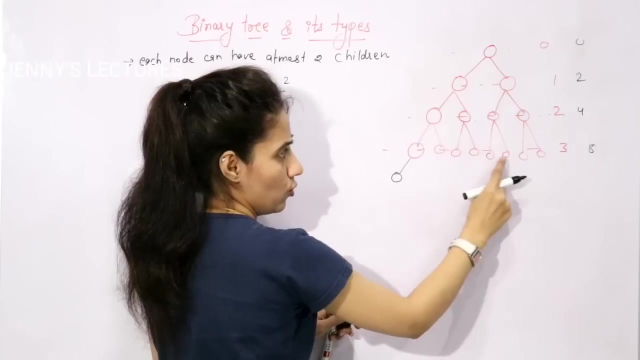 eight, right. so here eight can be possible, here four maximum, here two. here we can have zero, simply same. if I increase one level more, then here at this level, how many maximum number of nodes are possible? you can say each this, this node. at level three, each node will. 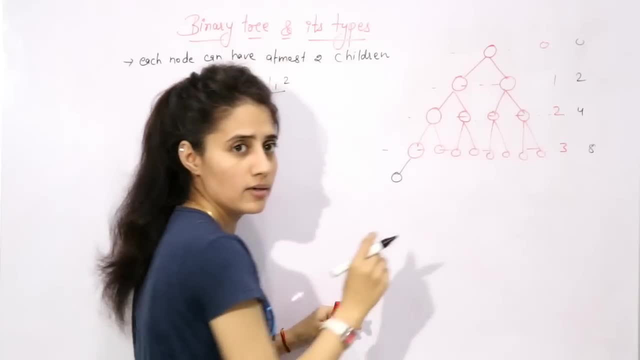 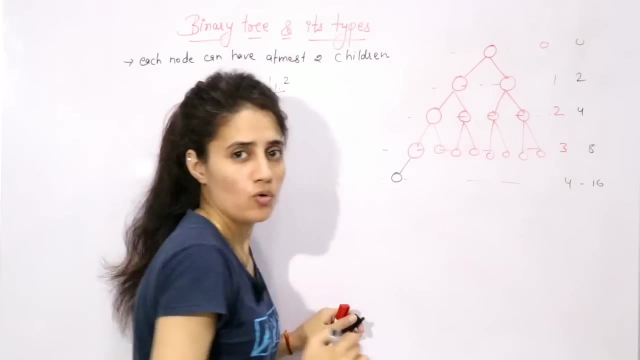 have two children. so here I have eight nodes. so eight into two, that is sixteen, can be possible. so at level four, sixteen maximum node can be possible. right now, how you can write this thing? can I write here two raised to power zero? can I write two raised to power zero? 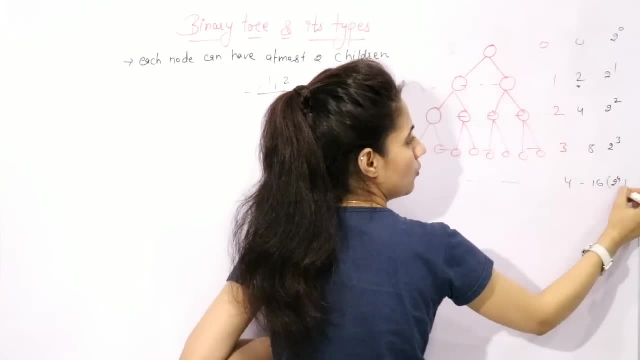 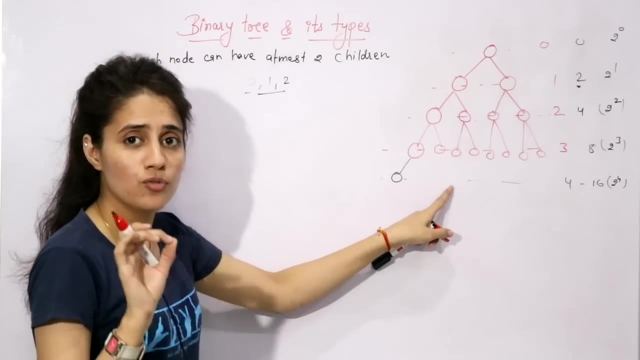 can I write: two raised to power one, two raised to power two, two raised to power three and two raised to power four. so now what you can say here at each level I. the maximum number of node possible in a binary tree is two raised to power. I. that is one property right, the. 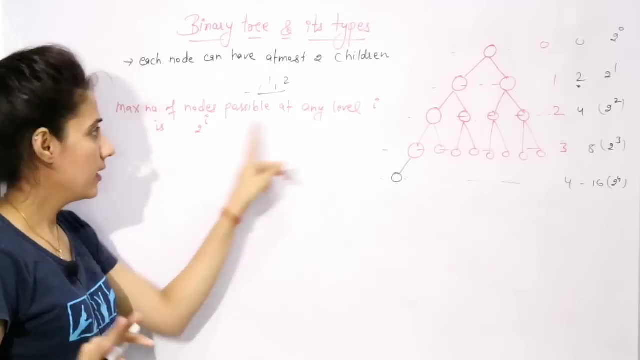 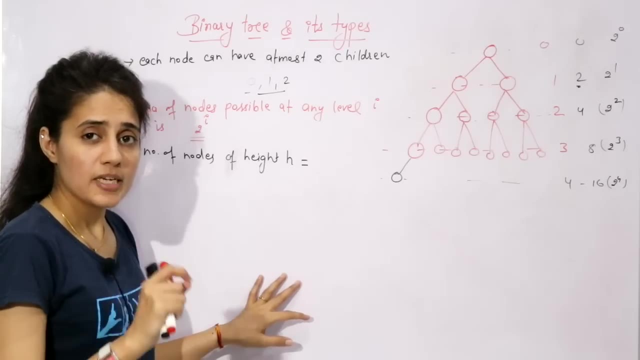 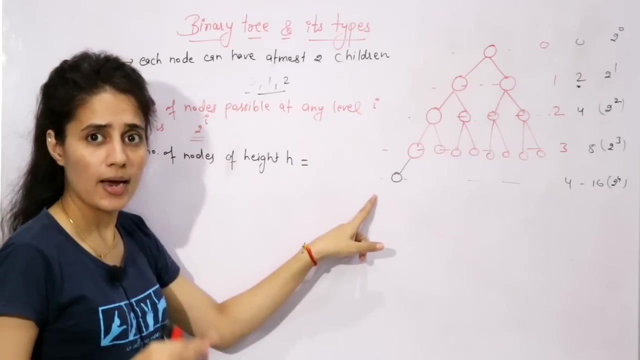 maximum number of nodes possible at any level. I is two raised to power. I right this thing. I have already shown you. now. next point may be the maximum number of nodes possible at height H, the maximum number of nodes of a binary tree right at height H. see at this. 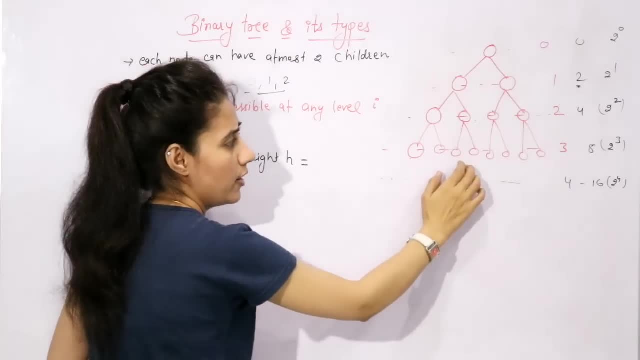 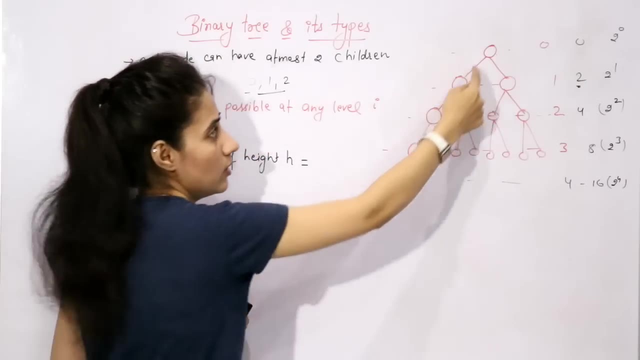 level. suppose I have three levels only now. height of this tree is what height of the root node is equal to height of the tree. height of root node is what one, two and three got to the longest path. find out the longest path, path from the root, or you can say from that. 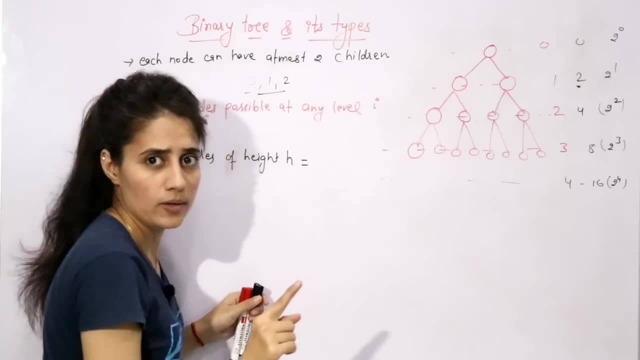 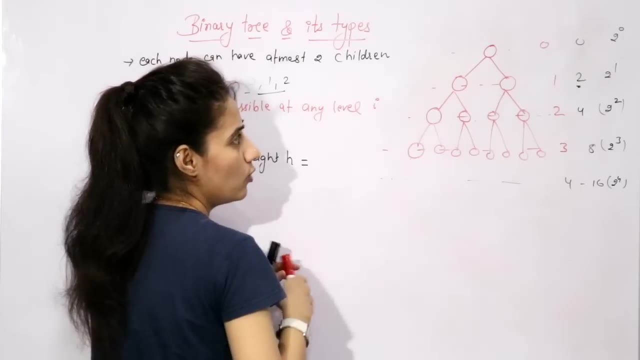 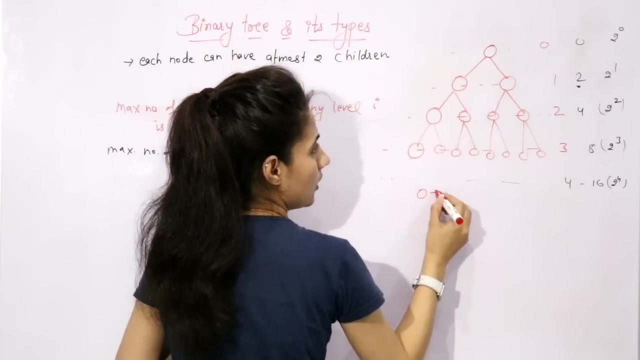 node to the leaf node. so now here, height is three. only right now, at height three, maximum number of nodes possible are: see how to calculate you are you are supposed to add all these nodes means you are supposed to add first of all 0 plus. at this level i have 2 plus. at this level i have. 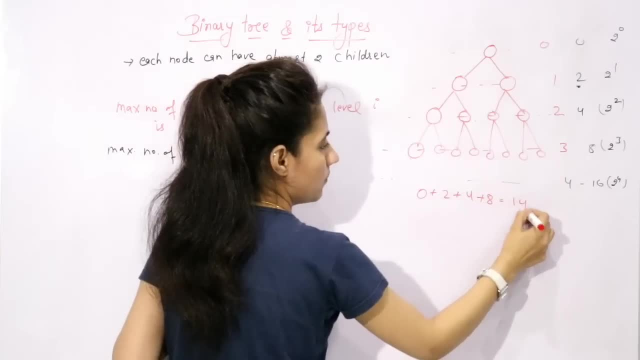 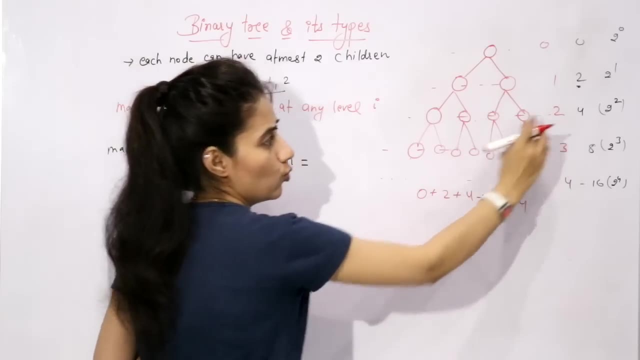 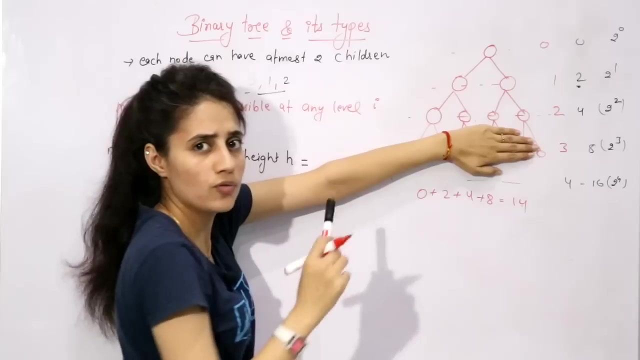 4 plus at this level i have 8. it means you can say 40 number of nodes: right, maximum number of nodes. fine. now if i say height is only 2, right, height is 2 means i am removing this level. means now height is 1 and 2. height of root is 2, so height of tree is also 2. now if height is 2 maximum number. 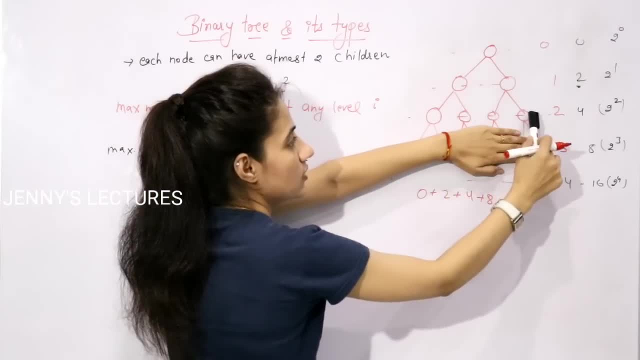 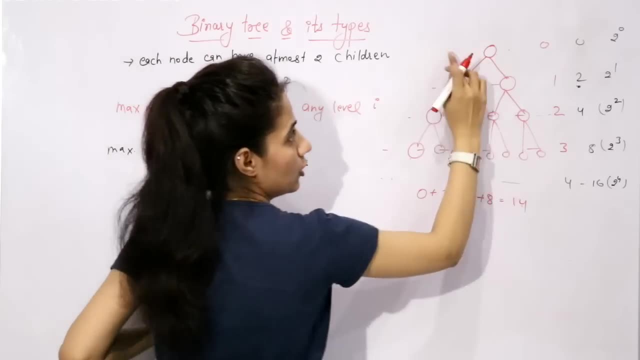 of nodes possible are 1, 2, 3, 4, 5, 6, 7. so how to calculate maximum number of nodes? if height is h, simply you will add all the maximum number of nodes at each level, so you can say 2 raised to. 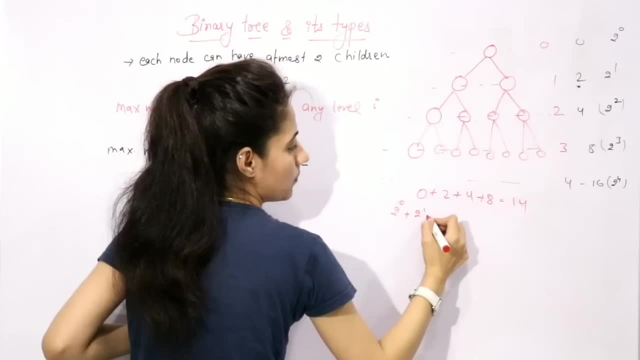 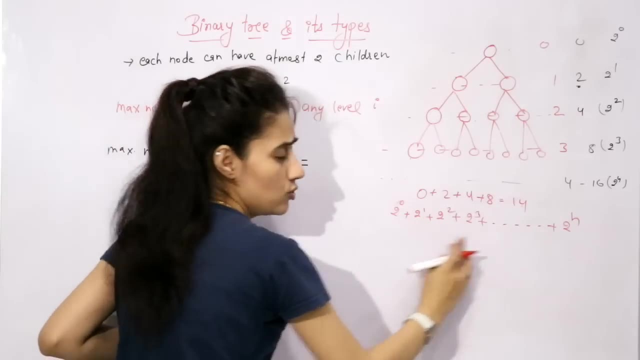 power 0 at this level, 2 raised to power 1 plus 2 raised to power 2 plus 2 raised to power 3 and till 2 raised to power h. ok, Now, this is what? simply a GP series and how to find out the sum. you can easily google it out. I. 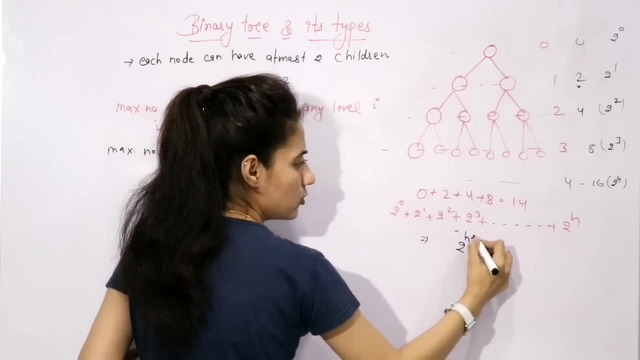 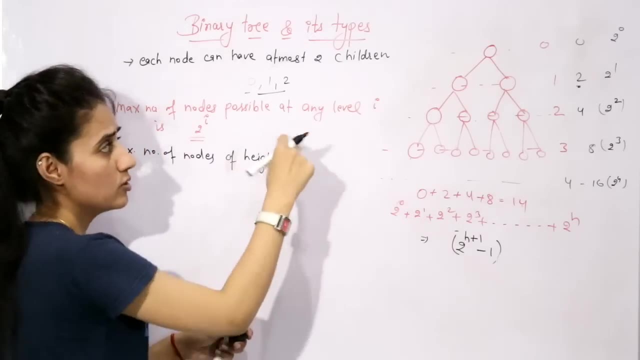 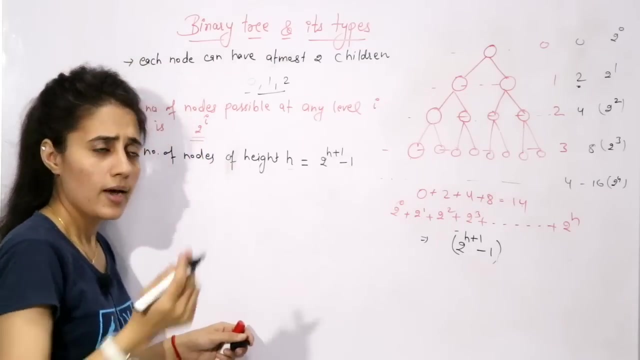 am not going to tell you this thing. So answer of this would be 2 raised to power, h plus 1 minus 1 right. So maximum number of nodes of height h- I am talking about this binary tree right. So maximum number of nodes can be h plus 1 minus 1 right. and if I ask you the minimum number of nodes, 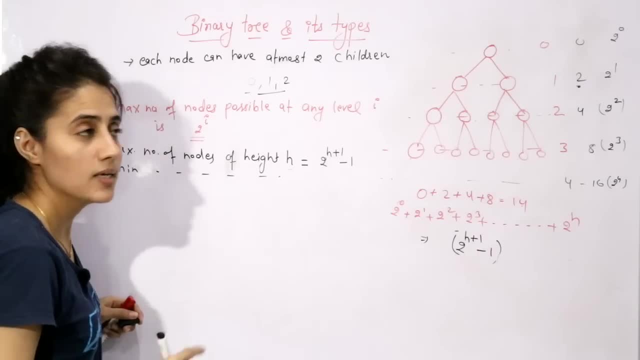 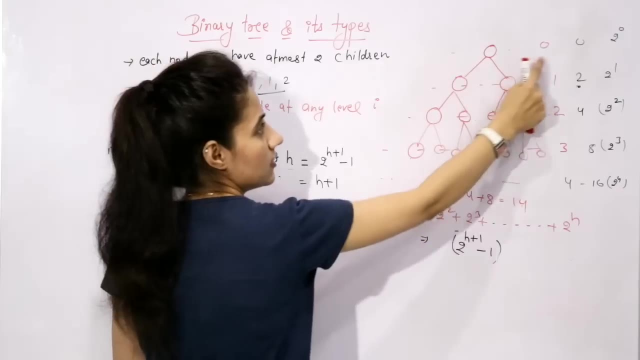 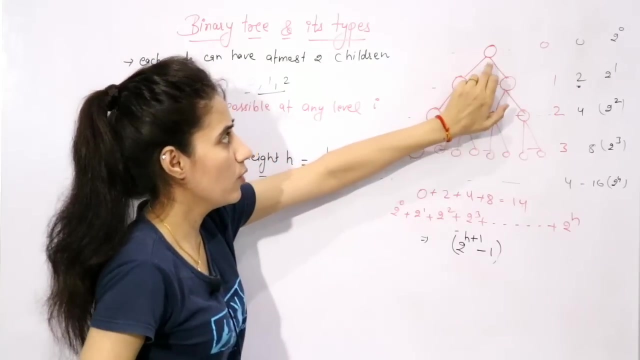 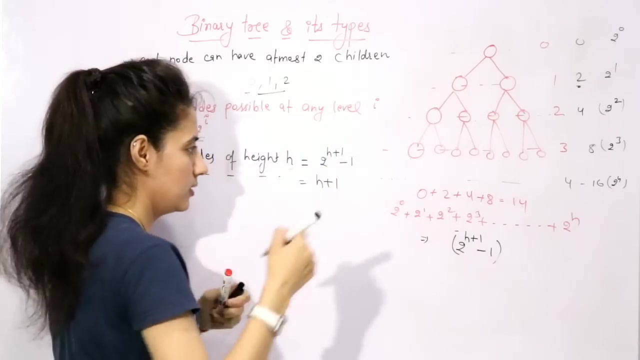 if height is h, then, see, minimum number of nodes can be h plus 1.. Now, if height is this one- 0, it means height is 0, means we have only one node. right, We don't have this thing. we have only one node. it means height is 0. So the minimum number of node is 1.. If height is 1, see, this is height. 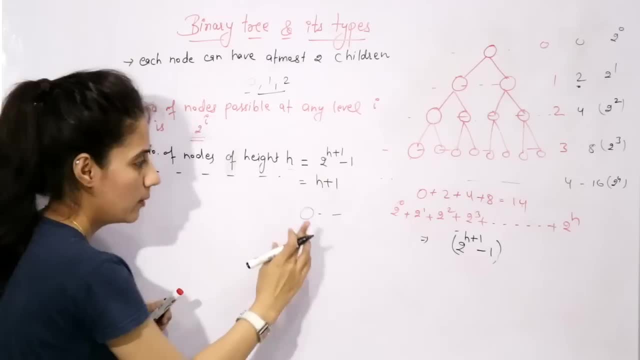 0. this is a tree, binary tree, having height 0. So if height is 1, then we have only one node, right? Minimum number of node is 1.. Now, if height is 1, I am going to increase the height. Now height is. 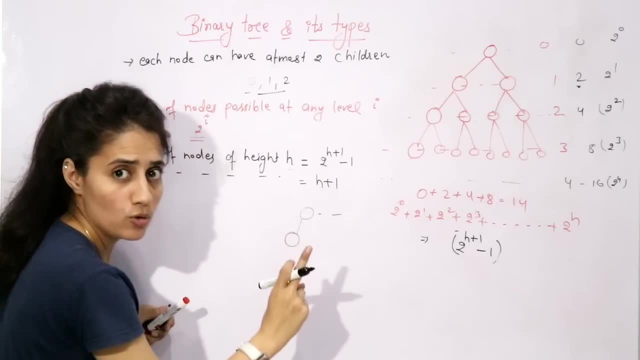 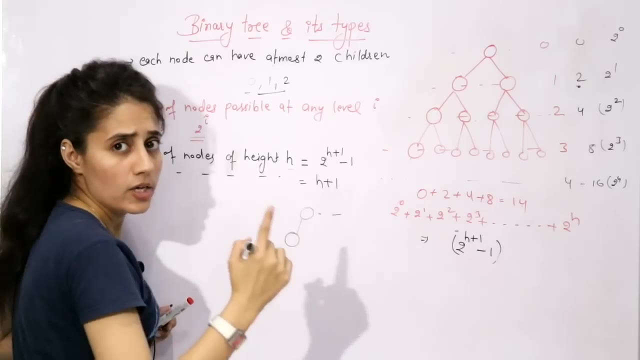 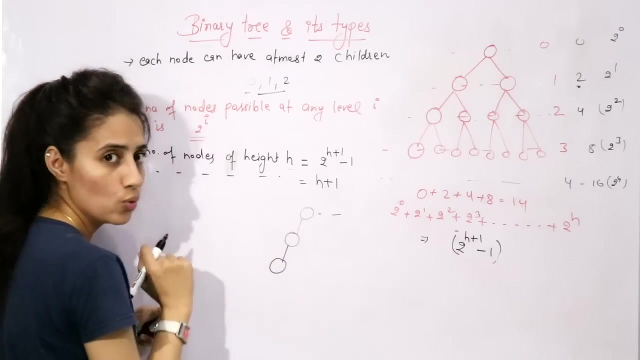 1. height of this tree is what? 1. Minimum number of nodes are 1 and 2, only Minimum number of nodes. I am not adding this node. second node: right Now, if you increase the height one more, suppose I am increasing height one more. Now height is 1 and 2. Now height is 2 and minimum number of nodes are 1. 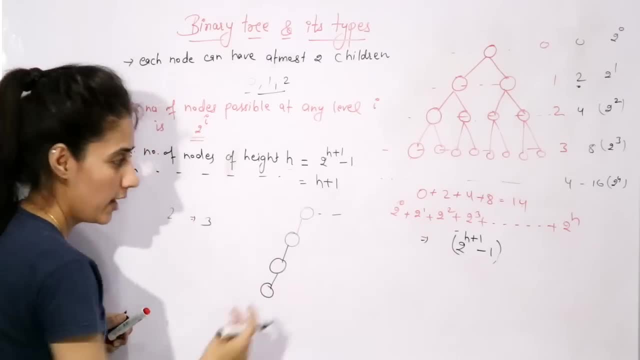 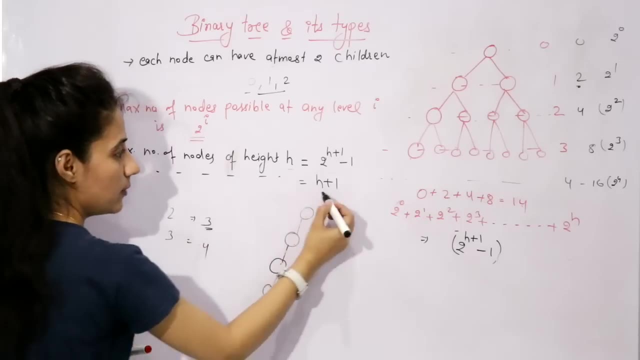 2 and 3.. If you will increase one more height, Now height is 1, 2 and 3.. Height is 3.. Minimum number of node possible are 1, 2, 3 and 4. So you can say minimum number of node possible are h plus 1.. h. 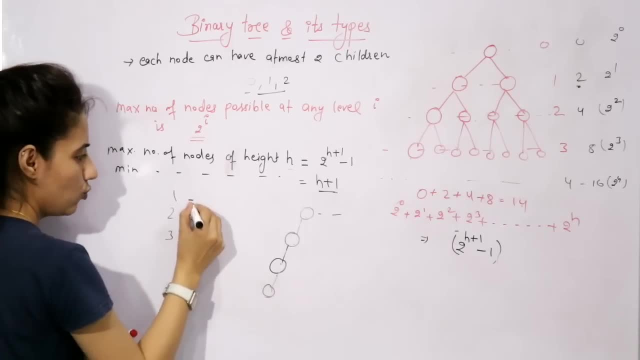 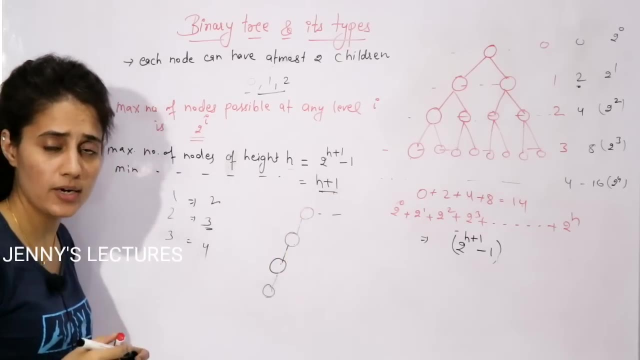 plus 1, h plus 1, 3 plus 1 is 4.. If height is 1, means this one, One height 1, 2. Two nodes are possible means h plus 1. Minimum number of nodes are possible right. Next thing is: if suppose you, 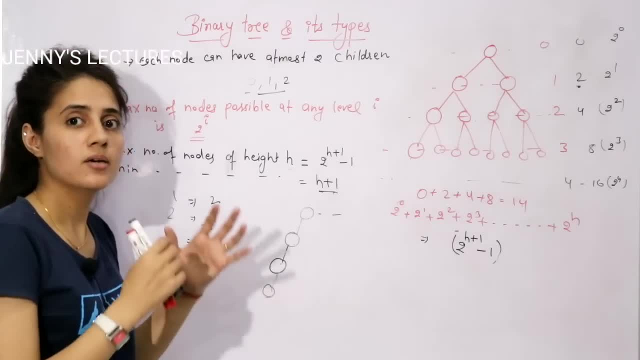 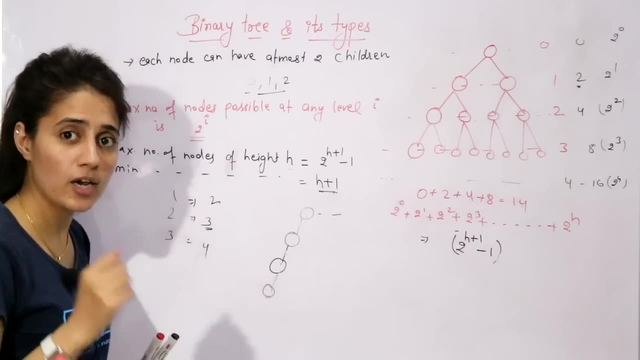 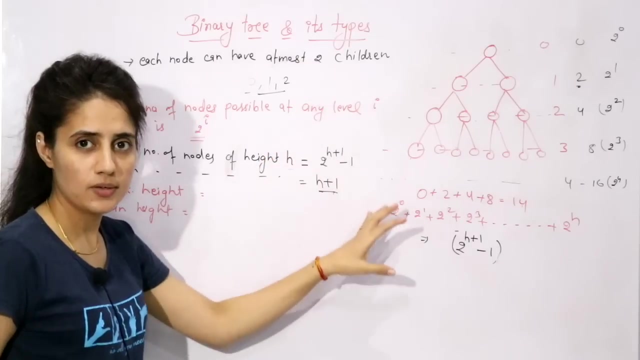 are given maximum node, minimum nodes, and you are supposed to calculate the height. You can say the maximum height of the tree possible and minimum height of the tree possible. Then how you will say, how you will calculate this thing? Now suppose you are given there can be n maximum nodes in the binary tree. Now you have to find out the possible height. 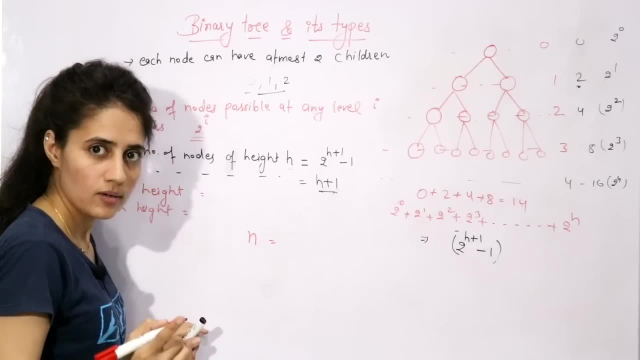 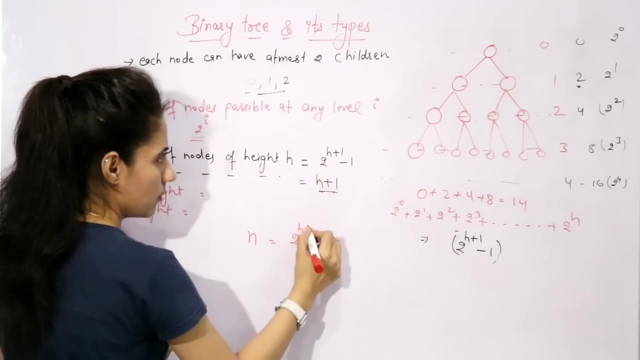 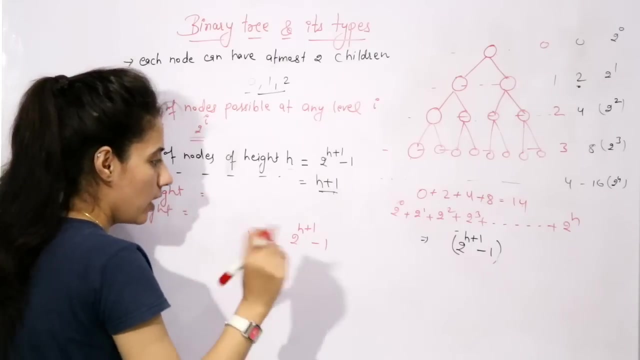 So maximum number of nodes are n. As from this case we can say: the maximum number of nodes can be of height. h can be 2 raised to power, h plus 1 minus 1.. Here you are supposed to calculate h value means. here I am calculating height of the tree. Now how you will. 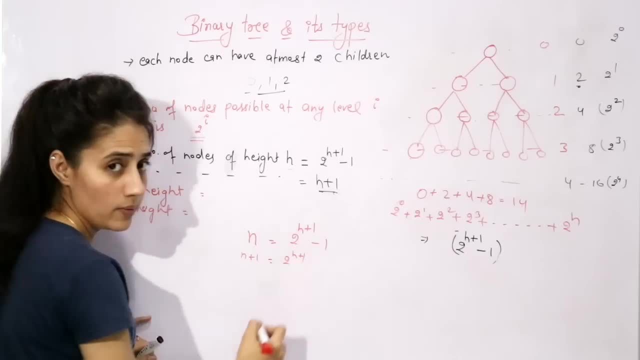 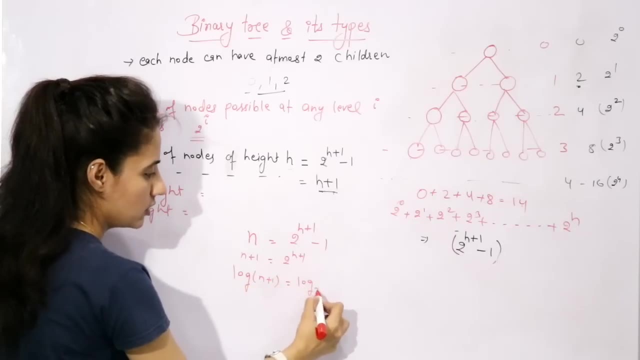 calculate: n plus 1 is equal to 2 raised to power h plus 1.. I guess you can easily solve this thing by taking log on both side, Log of n plus 1 and log of see. base is 2.. 2 raised to power h plus 1.. 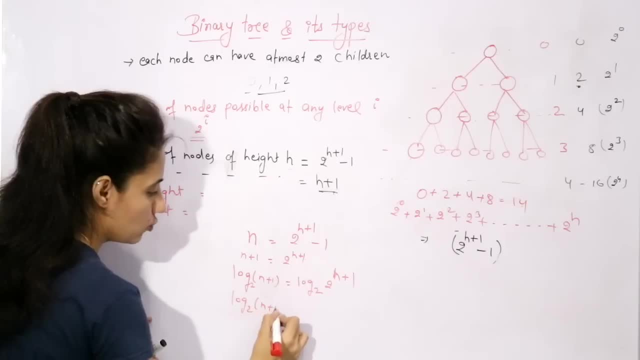 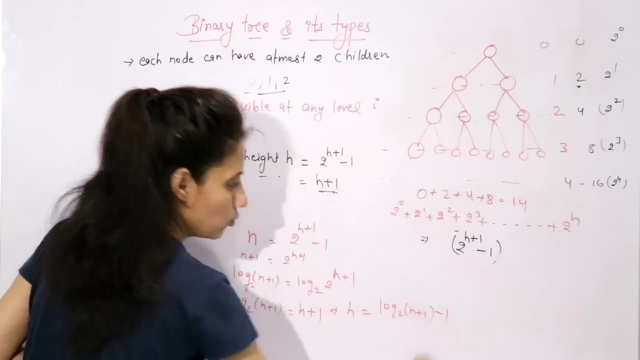 Now this thing is what? log 2 n plus 1, log 2, base 2 is this one, and this one is also 2.. So here you are supposed to calculate height. Now, here, height you are supposed to calculate height is equal to log 2 n plus 1 minus 1, and here we are taking the ceiling function. So this can be the 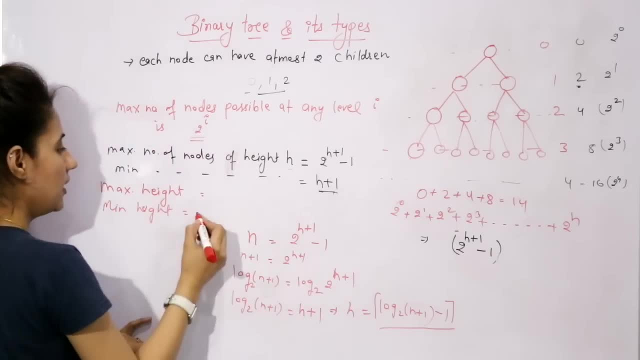 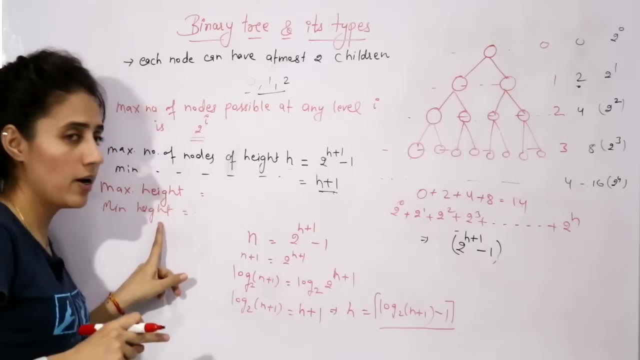 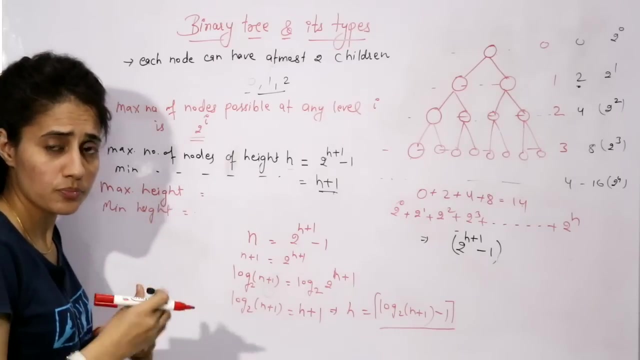 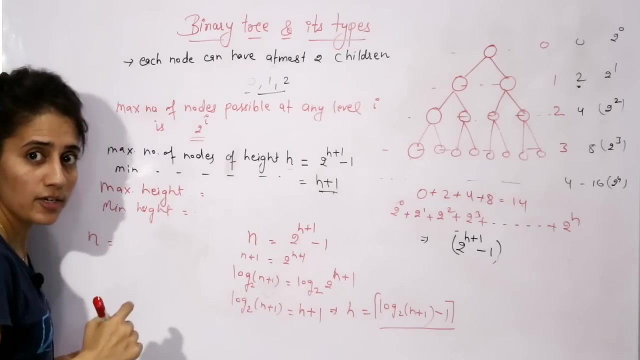 height. But this can be the minimum height. If maximum nodes are given. those nodes can find out using those nodes. you can find out the minimum height. If minimum number of nodes are given, that will give you the maximum height. Now, suppose minimum number of nodes are given n Now height. is what Now? minimum number of nodes. 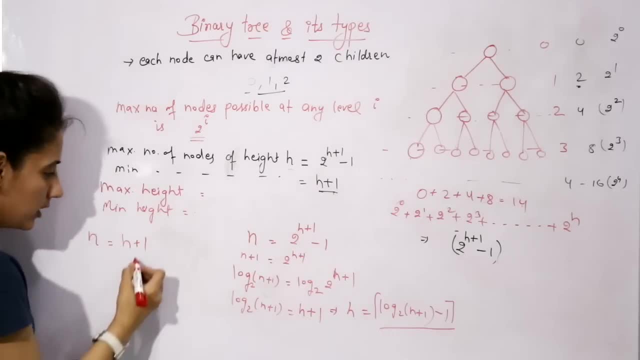 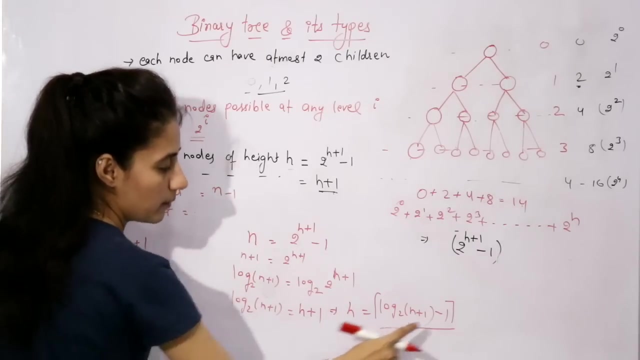 of height h. we know h plus 1 can be there. Now simply calculate the height is equal to n minus 1.. So this can be n minus 1, can be what? Maximum height- n minus 1- and minimum height can be this one log 2: n plus 1 minus 1.. Now we will see types of binary tree. 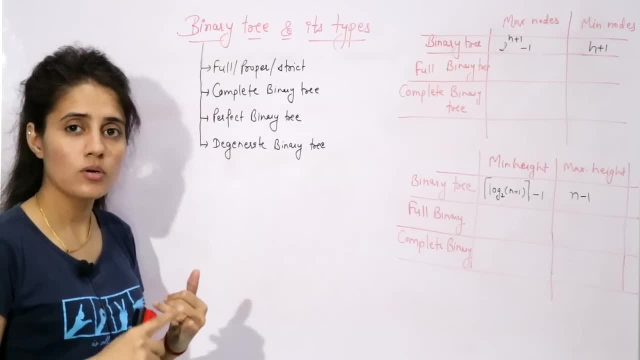 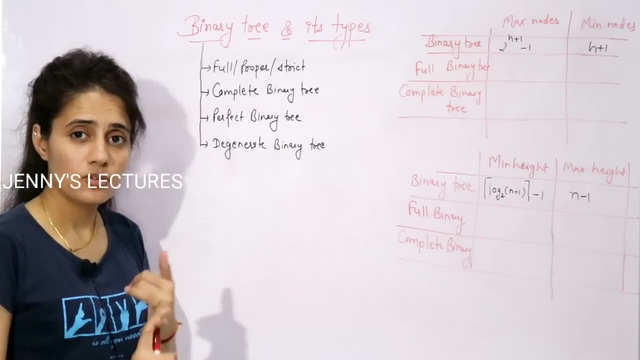 So types are: full binary tree- This is also known as proper or strict binary tree, complete binary tree, perfect binary tree, degenerate tree and balanced tree also. But balanced tree we will discuss when we will discuss the avial trees. right, That is also. that is basically known as. 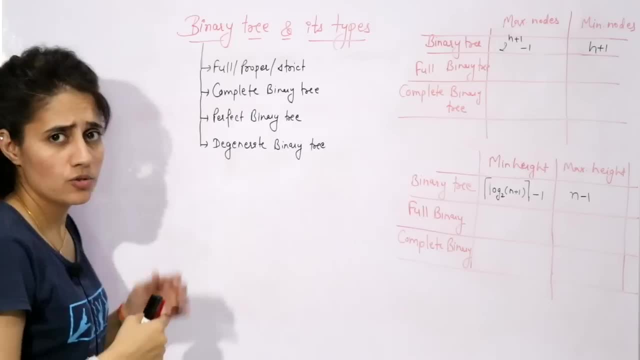 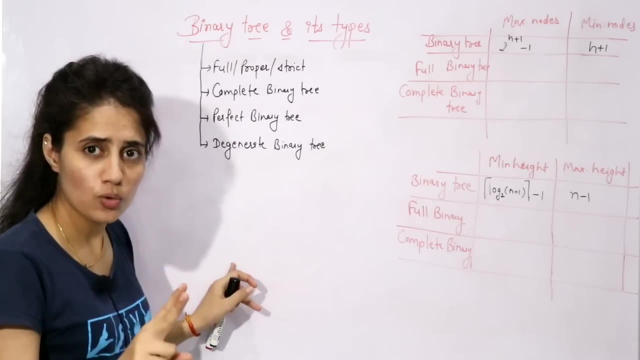 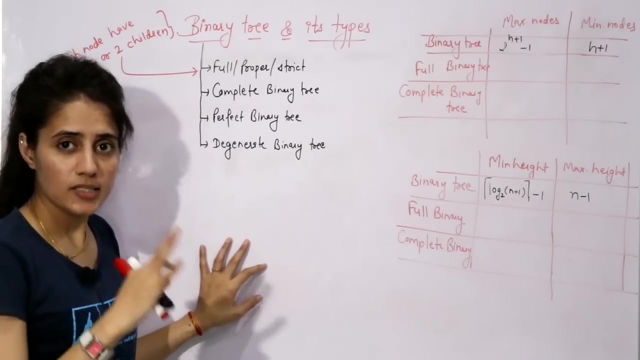 balanced tree. Now, what is full or strict or proper? binary tree? See, the definition is what It is: a binary tree where each node contains either 0 or 2 children, or in another term, you can say: it is a binary tree. See, obviously it is a binary tree. 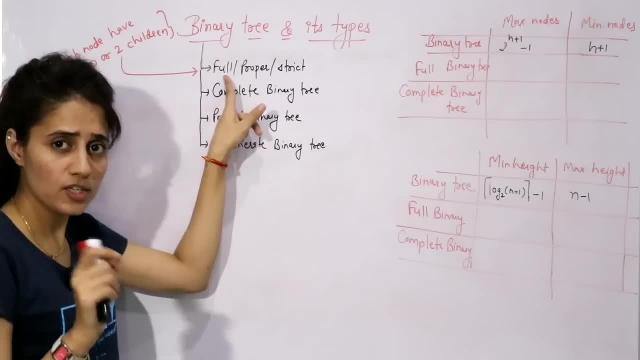 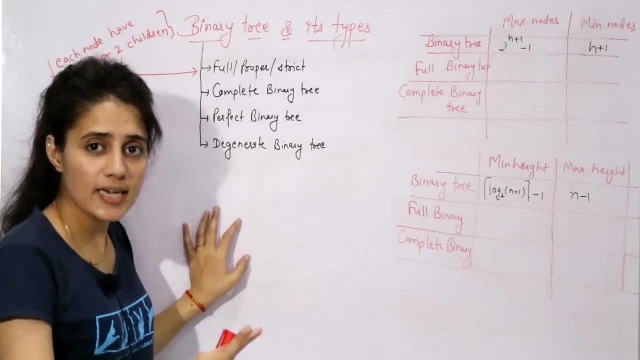 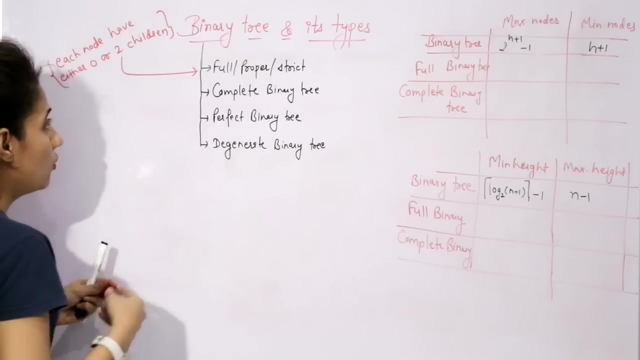 plus. one more condition is it is each node is containing either 0 or 2 children, or you can say each node will contain exactly 2 children, except leaf node. right Now, see what is a full binary tree. Now, if I draw something like this: 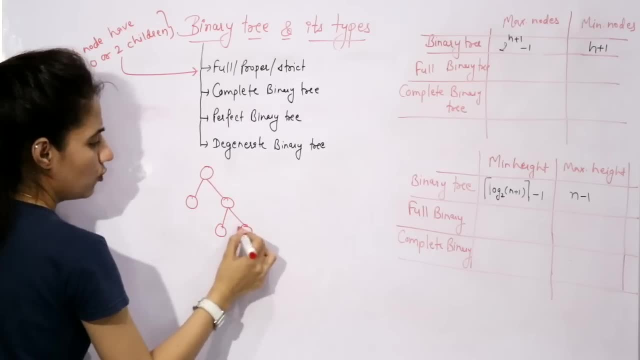 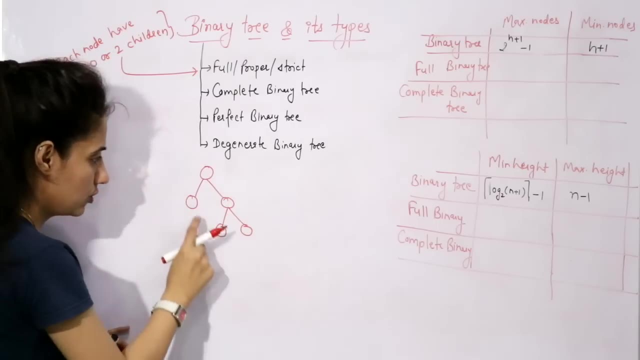 Now choose this. Is it a full binary tree? Yes, because it is a, first of all, a binary tree. plus, here each node is containing either zero- see, this one is containing 0,, 0, and 0 means these are leaf node right- or 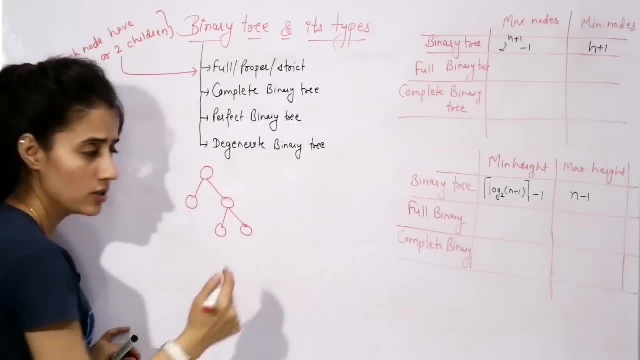 2 children. This is containing 2 children. This is having 2 children. So this is what a full binary tree. Now see, this is what. Is this? a full binary tree? No, this is not Why. so, because this node is. 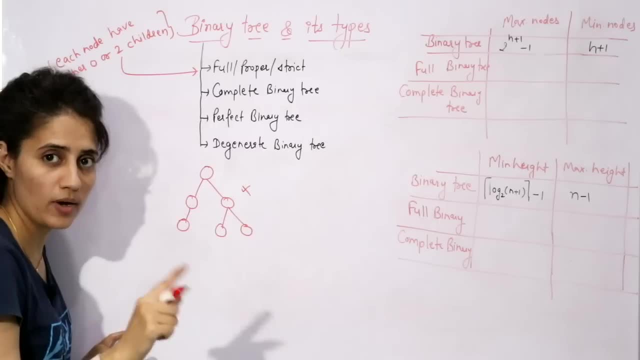 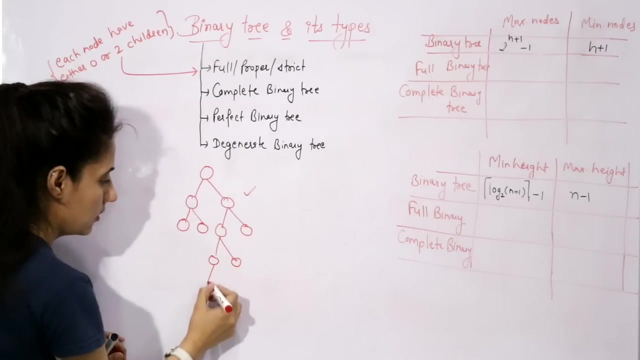 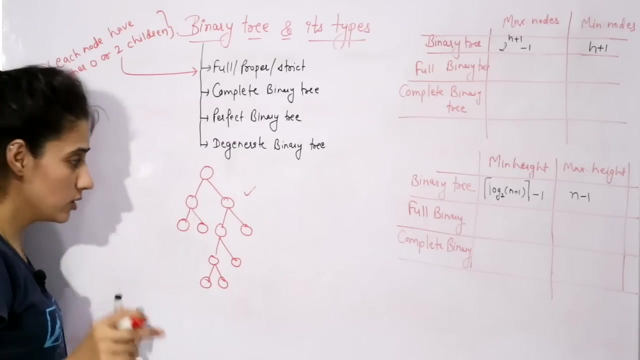 having only one child, But is not possible in full binary tree. now see this is what? is this a full binary tree? yes, this is a full binary tree right now. see, is this a full binary tree? yes, it is a full binary tree. is this a full binary tree? no, but is this a full binary tree? yes, each node is containing either zero or 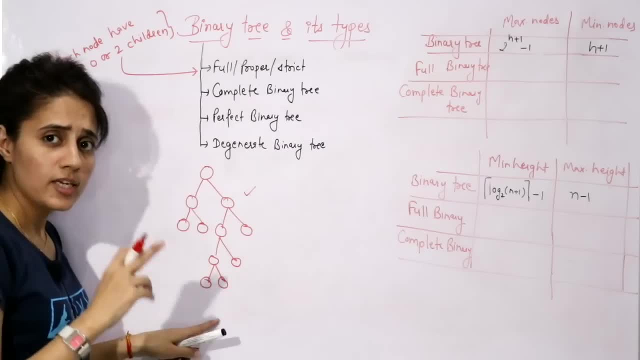 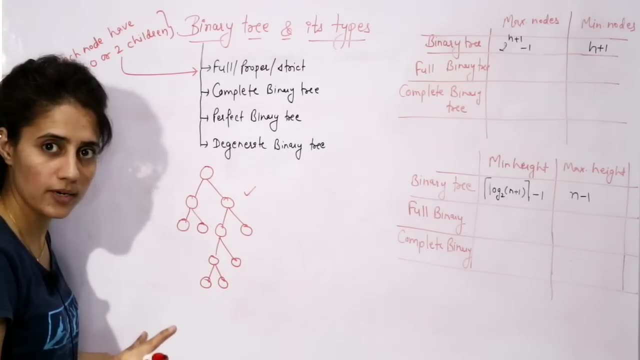 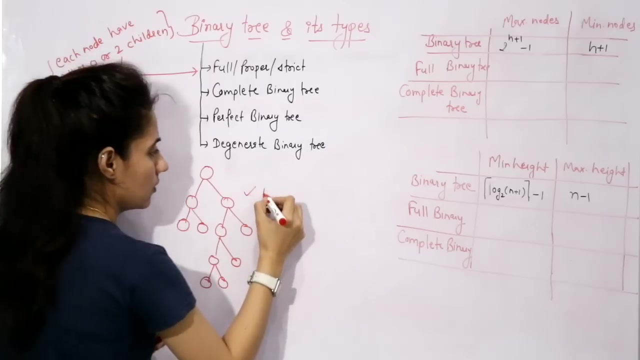 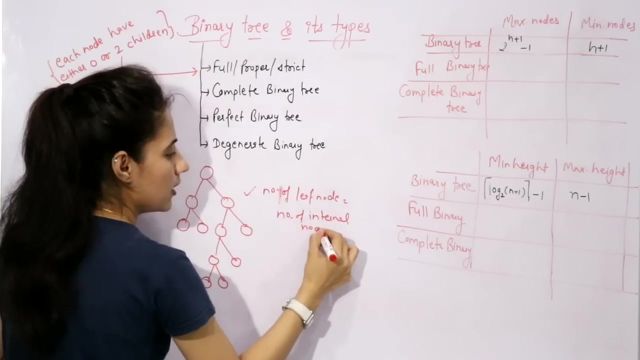 two children or all the nodes are containing. each node will contain exactly two children, except leaf nodes, except leaf nodes, right now same. the property of this full binary tree is what? here number of leaf node is equal to number of internal nodes plus one. here you can say this is a full binary tree. now, here number of leaf node count. 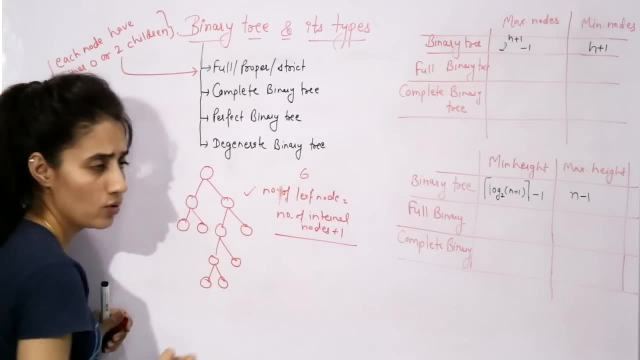 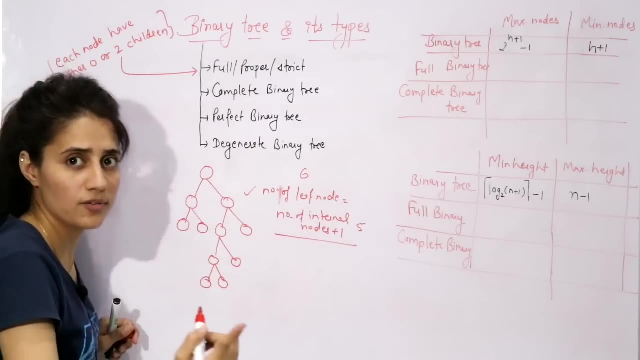 one, two, three, four, five and six. number of leaf node are six. right it should be equal to number of internal node plus one means here number of internal node should be five. one, two, three, four and five. i have discussed what is leaf node, what is internal node in the previous 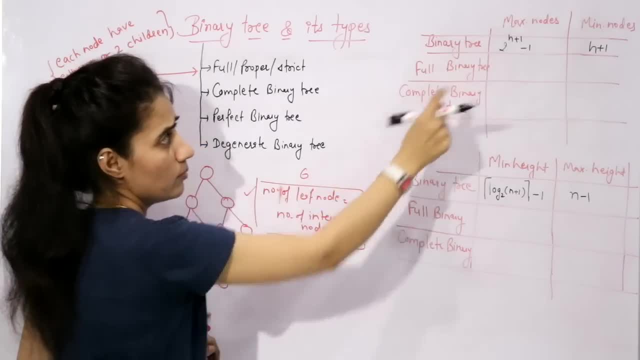 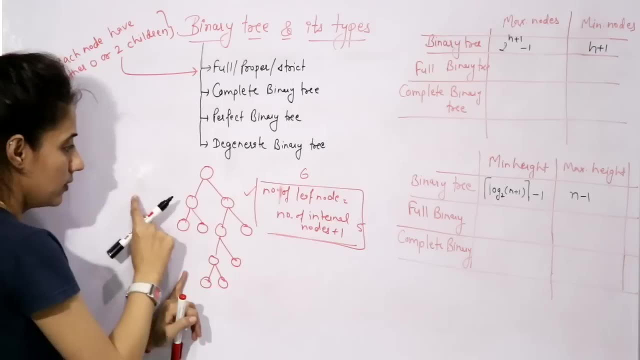 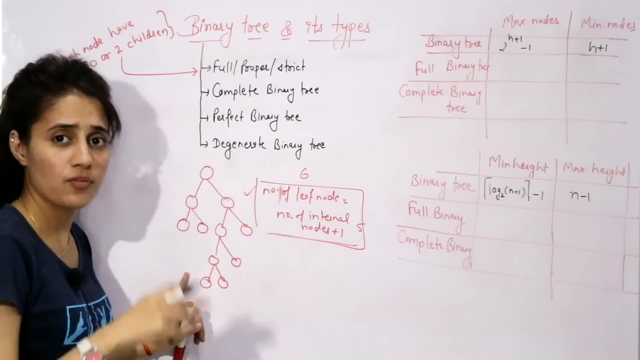 video. you can check out that video if you don't know. now, what about maximum node and minimum node in this tree? see, maximum node is same as binary tree. right, because here, also at this level, at this level. at this level means at every level i, there can be two raised to power, i maximum nodes. and if height is at h, then you need: 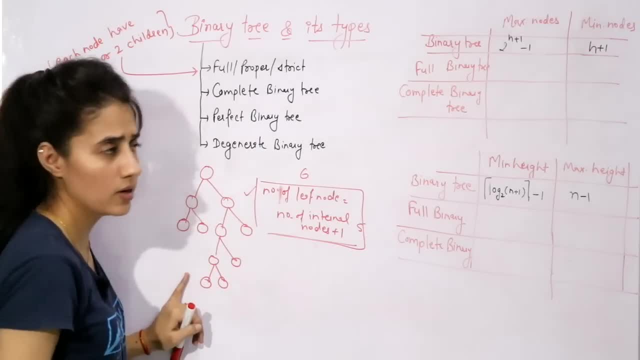 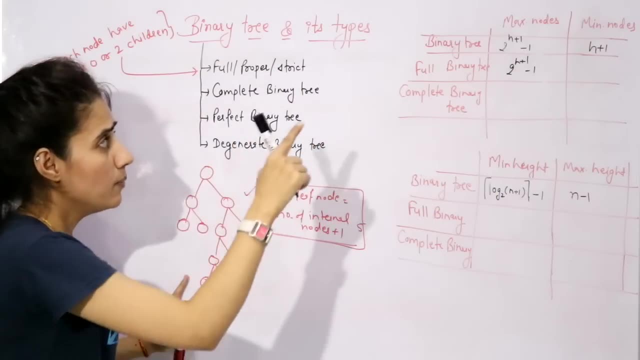 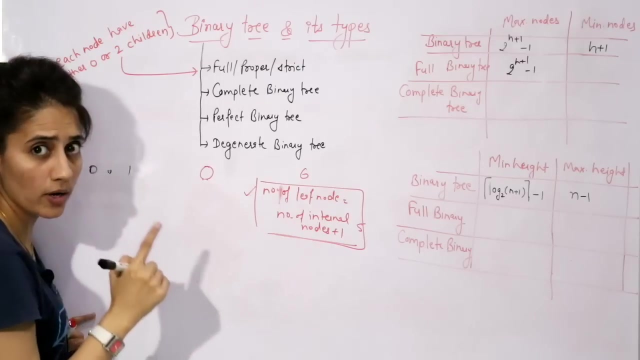 to add all the maximum number of nodes at each level. so this is two raised to power h plus one minus one. this thing we have already discussed right now. what about minimum nodes? see the minimum number of nodes. height is one, sorry, height is zero. so minimum number of node can be one. 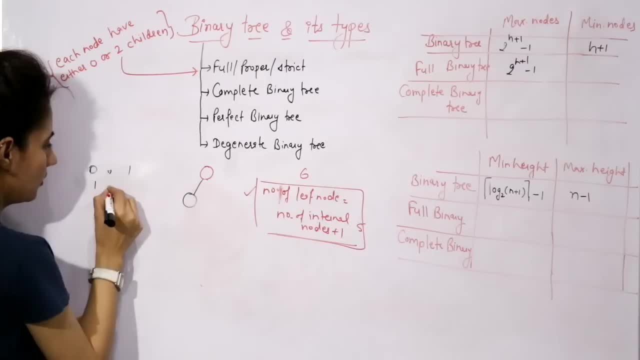 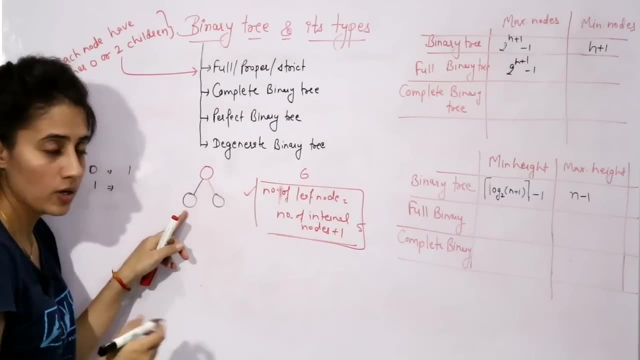 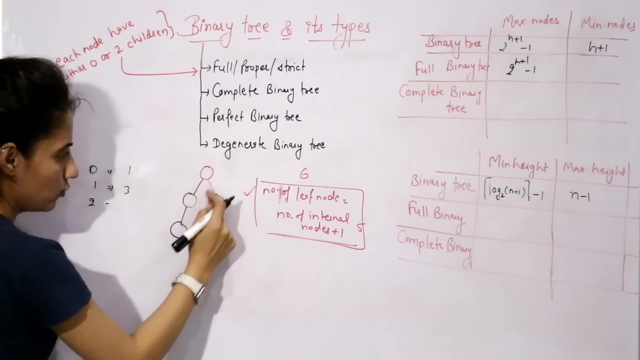 if i am increasing height one, this is height one. so minimum number of node can be three and three. Lusty student, how you know. one number of nodes, five and six. so that's it. now, what is mutual node? this is surely not a full binary tree, your maximum. 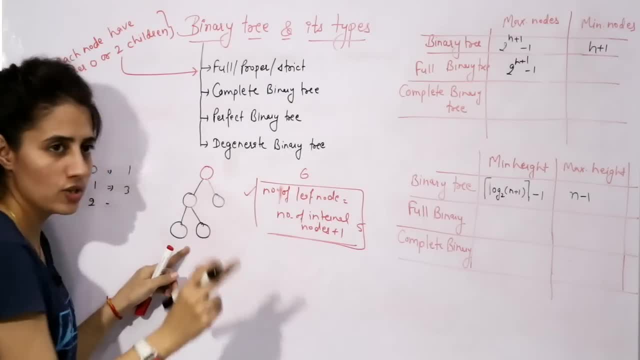 number of nodes. it means it is a single binary tree. that's all you need to know. while analyzed, when you see three, this is not a full binary tree. we need a full binary tree. so here you need one more node. so three can be the minimum number of nodes. now, if you increase height one more time, that is. 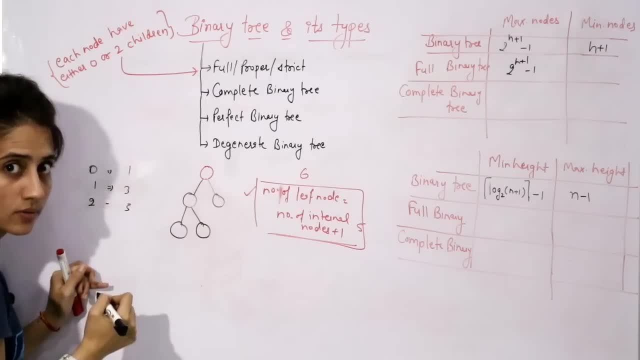 now, height is one and two. height of this tree is two, but this is not a full binary tree. you So 1,, 2,, 3,, 4,, 5,, 5, right, If height is 3, I am increasing one more height: 1,, 2 and 3.. Here also you need 2 nodes, So minimum number of nodes can be plus 2, that is, 5 plus 2 is C. So now how you can write down this thing: See 2 raised to power h plus 1, minimum number of nodes. 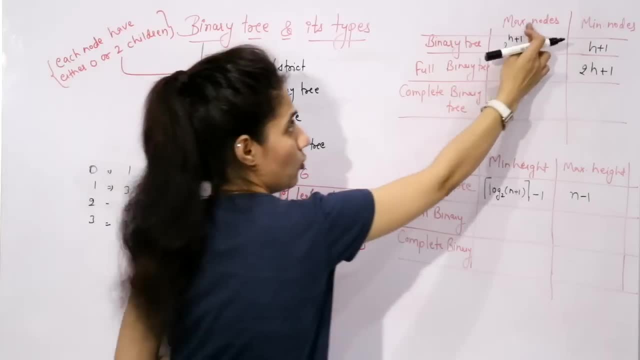 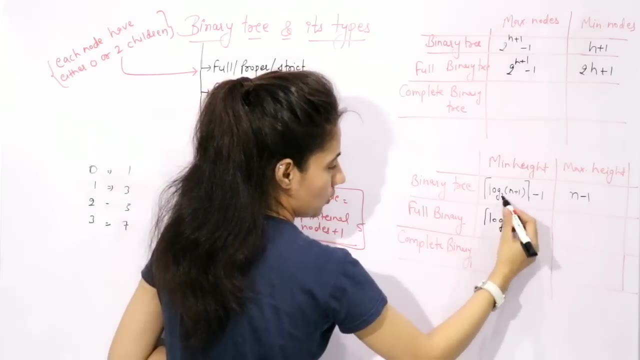 Now how to calculate minimum height and maximum height. See the maximum nodes will give you minimum height, this one minimum height. So minimum height would be same as previous one as binary tree: n plus 1, here ceiling minus 1, right. 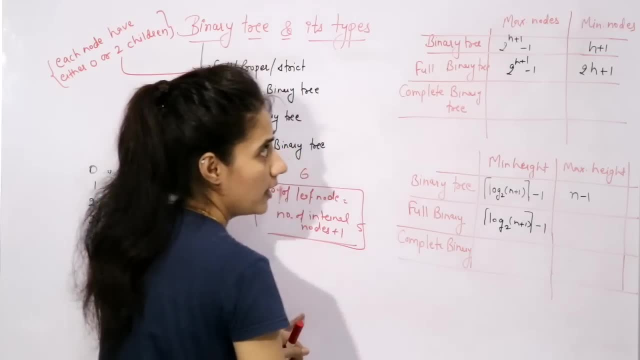 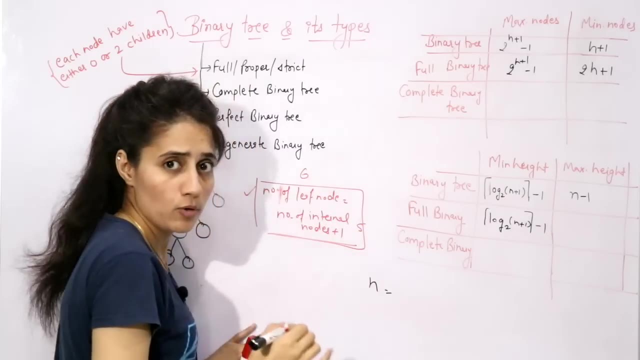 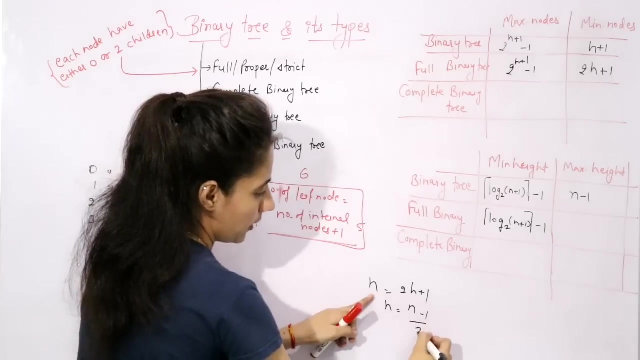 Because maximum node are same, But here the maximum height can be. the minimum nodes are 2 raised to power, 2 into h plus 1.. So how to calculate if minimum number of nodes are given n? how to calculate height? 2h plus 1, h is equal to n minus 1, divide by 2.. 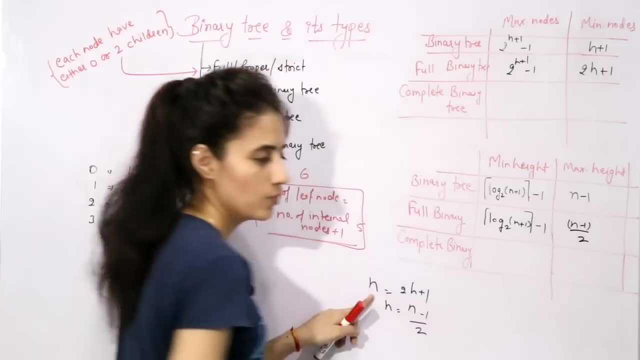 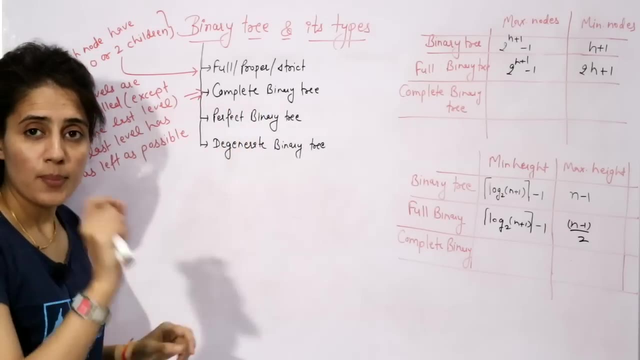 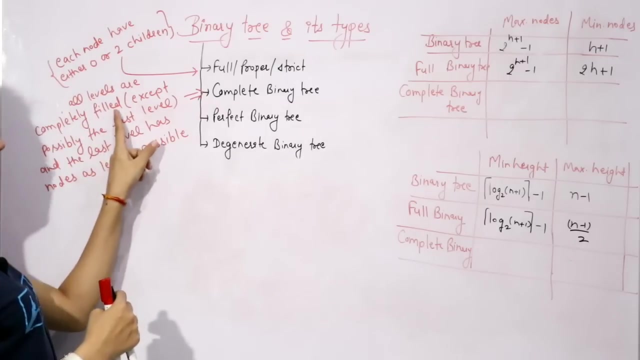 So here you write: n minus 1 divided by 2.. Now, next is complete binary tree. So now, according to the definition of a complete binary tree, See, a binary tree is a complete binary tree If all the levels are completely filled. all the levels are completely filled, except possibly the last level. 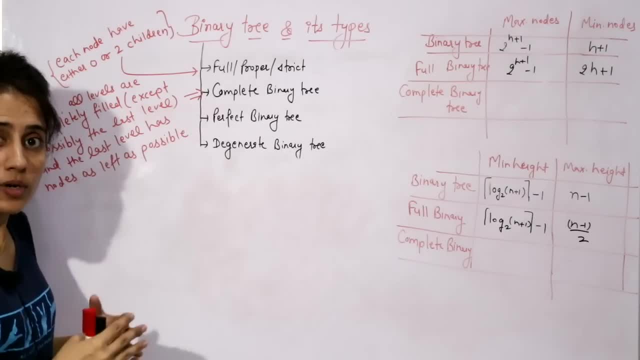 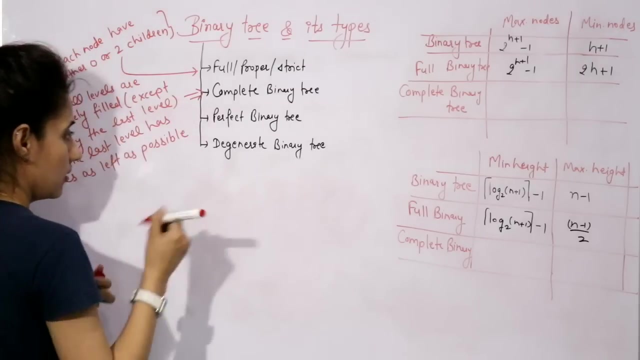 Fine Plus at the last level. we have one more condition, See, and the last level has the nodes as left as possible. Right, We are going to fill the last level from left to right, See. now I am going to take one example. 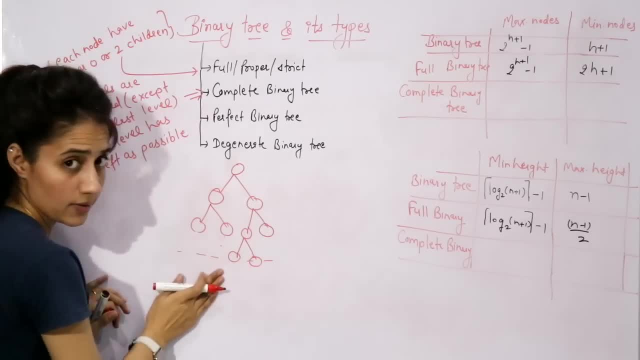 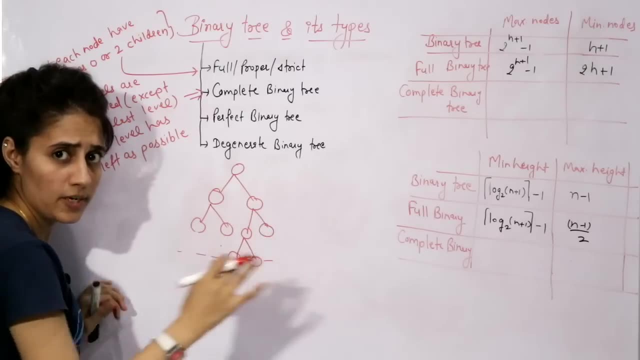 See, here, this is the last level right, And this is not completely filled because these nodes are not having any child. So that is fine in complete binary tree. See, we have told you, I have told you, except the, possibly the last level. 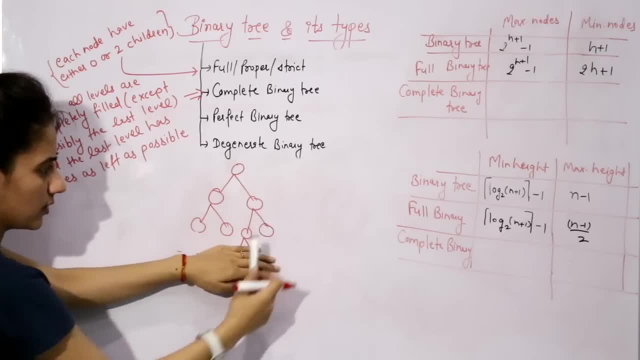 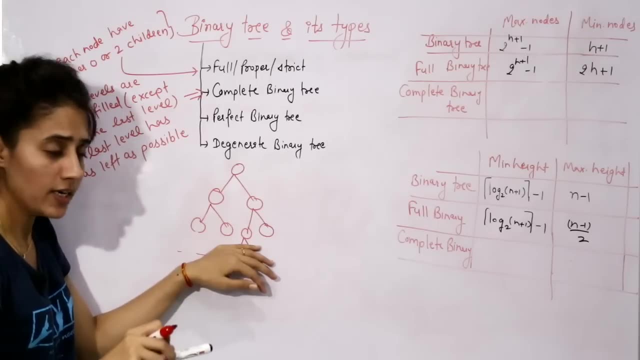 All the levels are completely filled. See now this level, this level, this level. This is what completely filled Right Each node is having two child. So one condition is true. Now, second condition is complete binary tree is what? 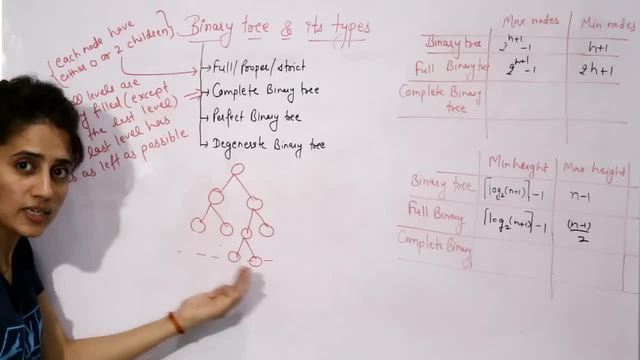 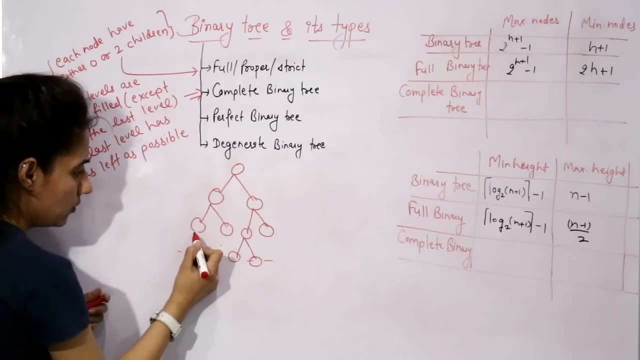 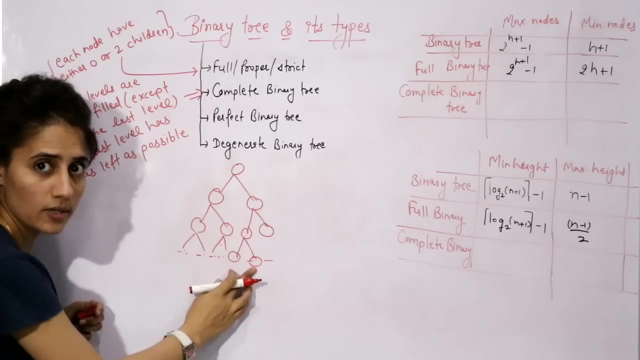 In the last level. the nodes should be as left as possible Means we are going to fill the nodes in the last level from left to right. You cannot leave these nodes free, these spaces free, and you cannot write here the child node. 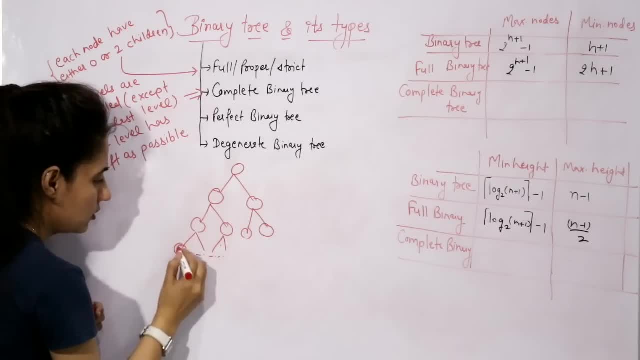 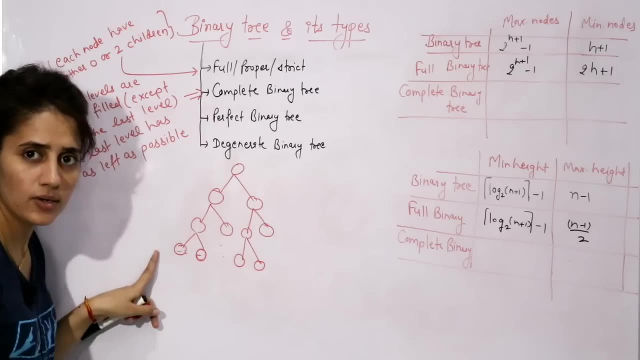 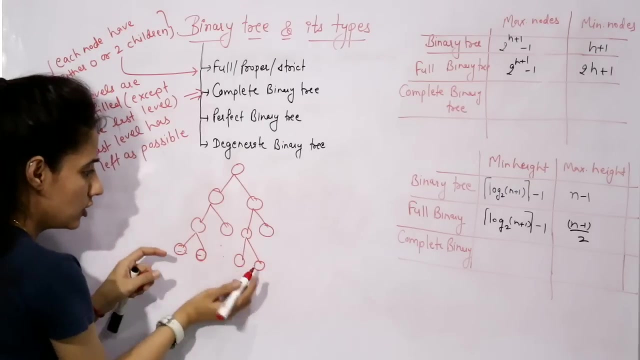 Right, You need to delete, and if I shift here, then this is what a complete binary tree. Now, is this a complete binary tree? No, Why? so See, except the last level, all the nodes are completely filled. But second condition is what? 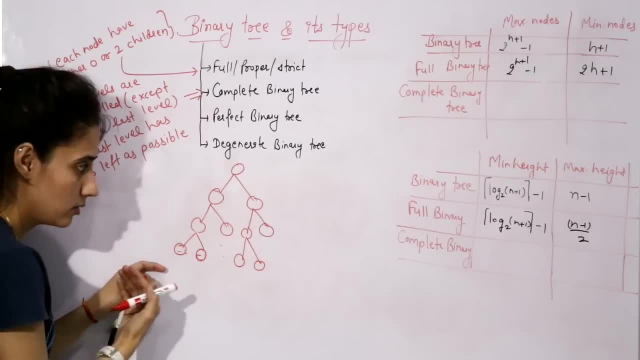 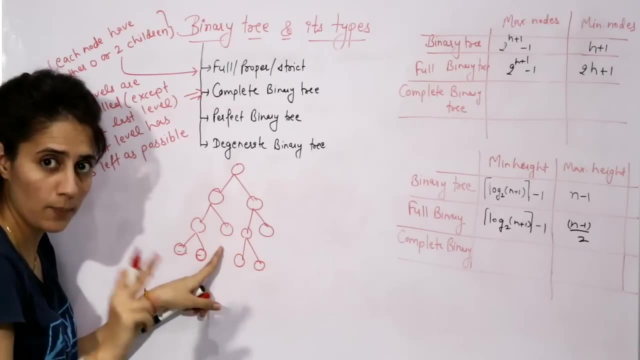 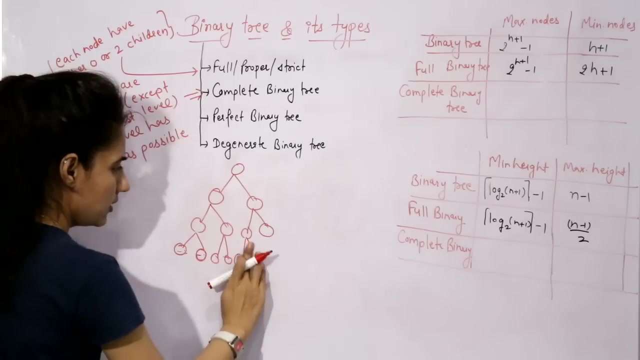 Here the nodes should be as left as possible. We have left this node blank and we have put children to this node. That is not true in complete binary tree. If this is also having two child, then this is fine. Right Now, is this a complete binary tree? 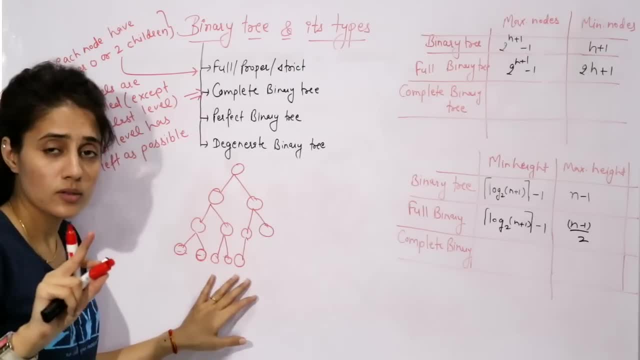 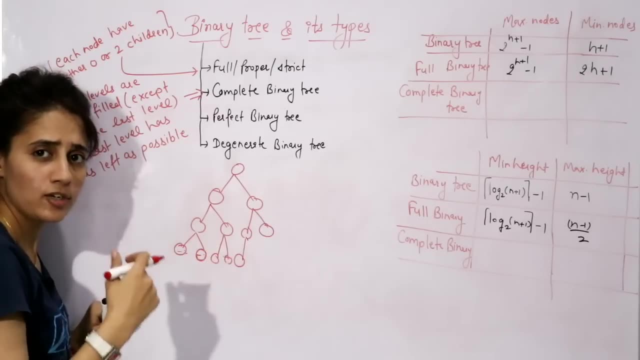 Yes, Because here the condition is not that each node is going to have exactly two children. So at the last level you can have one child, But that should be filled from left to right. See here, if you write this thing, you cannot fill the right child. 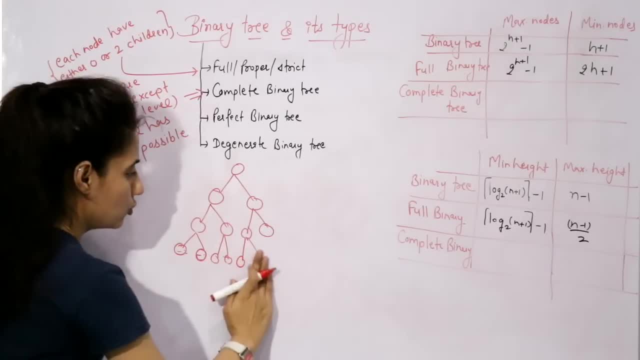 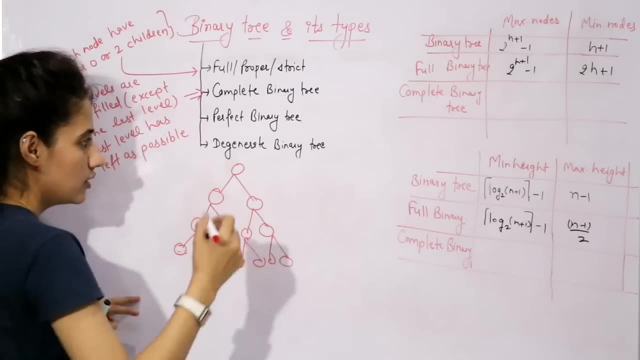 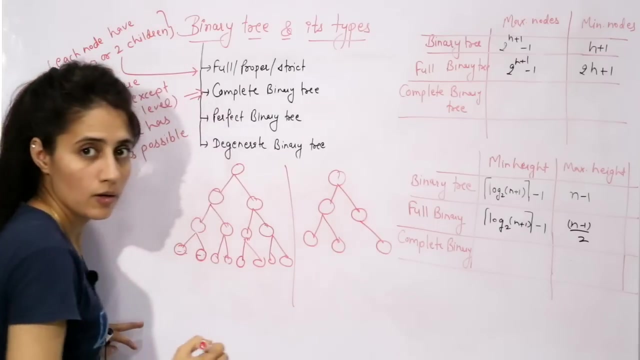 First of all, you will have to fill the left child Right. So now this is also a complete binary tree Right, And this is also a complete binary tree. Now see, is this a complete binary tree? No, this is not. 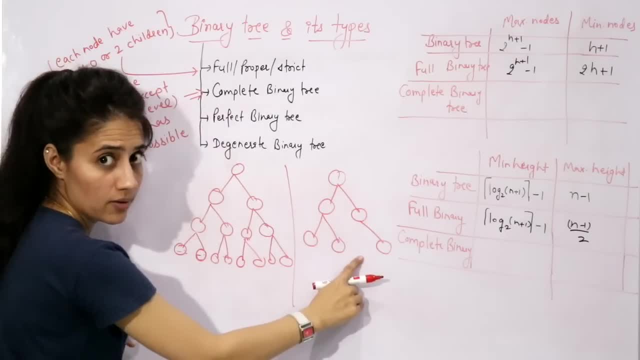 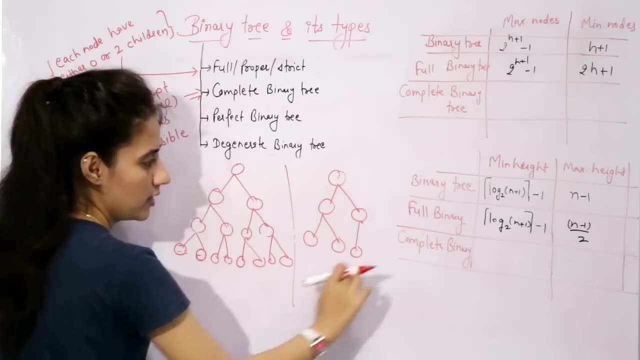 Because now this is the last level, Right. So at the last level you can fill the node from left only. So here you should fill the left child. You cannot fill first of all the right child. Is this the complete binary tree? 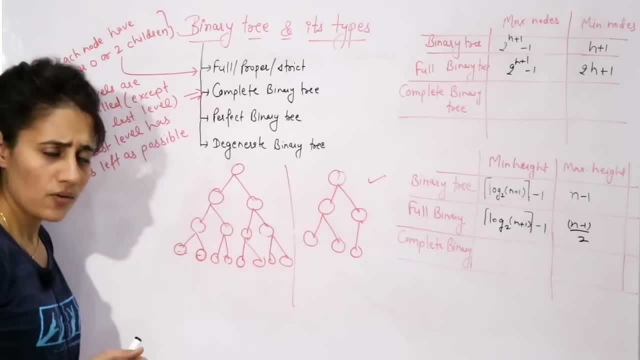 Yes, this is a complete binary tree Right. Somewhere it is also written, as it is nearly complete binary tree Right Now. in this case, also same. What about maximum node and minimum nodes? Maximum node: obviously this is a binary tree. So maximum node are same, that is, 2 raised to power h plus 1 minus 1.. Maximum node in a complete binary tree of height h. Right Now, what about minimum number of nodes? Here? the minimum number of nodes are 2 raised to power h. 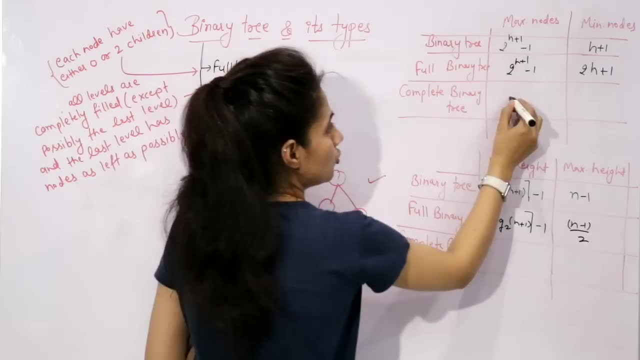 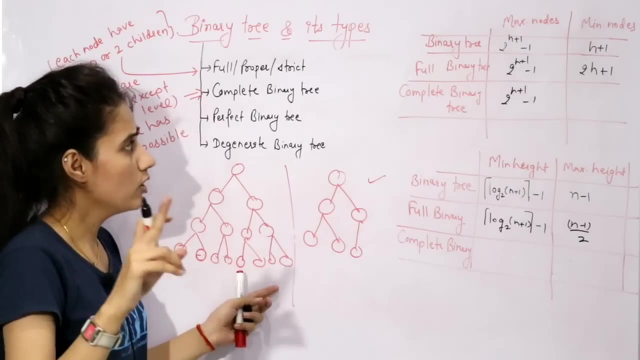 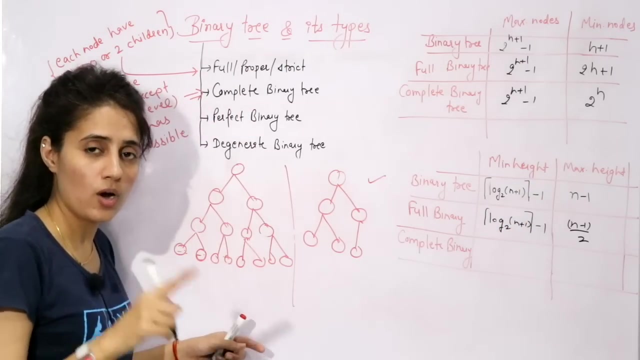 This thing: you need to find out how the number of minimum number of nodes are 2 raised to power h. I am not going to trace out the number of nodes, I am going to trace out this thing Now: minimum height and maximum height. Obviously, minimum height would be same as the previous one, because maximum nodes are same in all the 3 binary trees. Right Now, what is maximum height? Maximum height means minimum nodes will return you the maximum height. So how you will calculate? 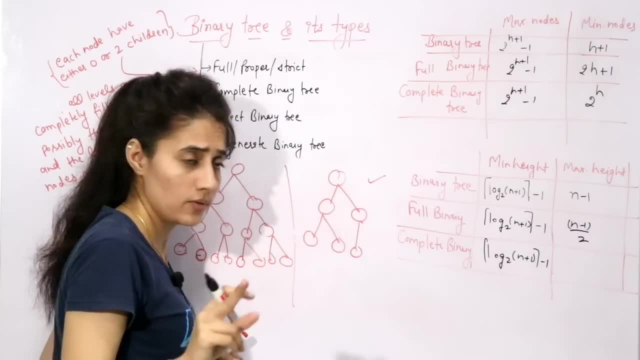 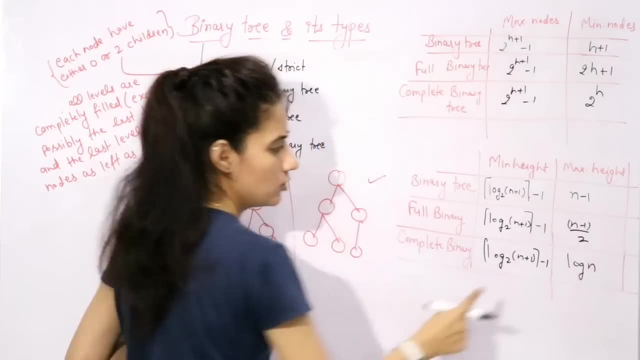 I am going to write down this thing. You need to calculate this thing Right. So the minimum height, Minimum height, Minimum height, So the minimum- sorry, the maximum height in a complete binary tree is log n. This thing you need to calculate how this is 2 raised to power h and how this is log. 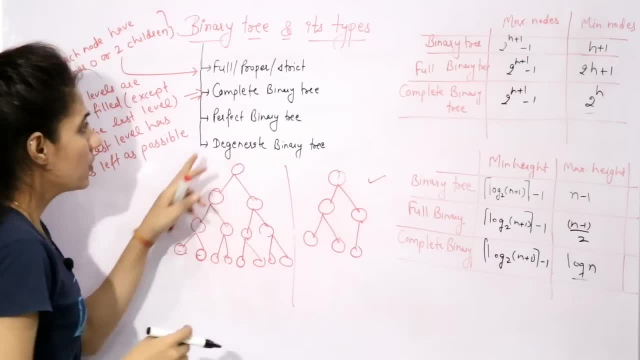 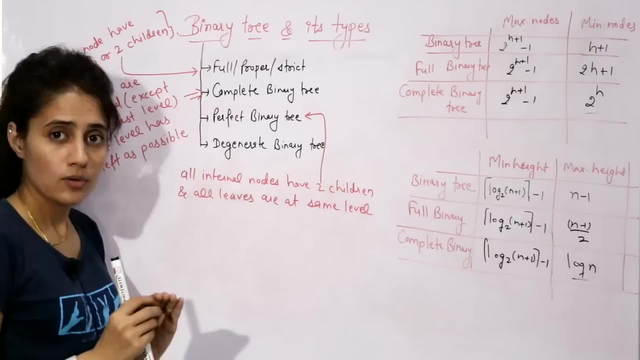 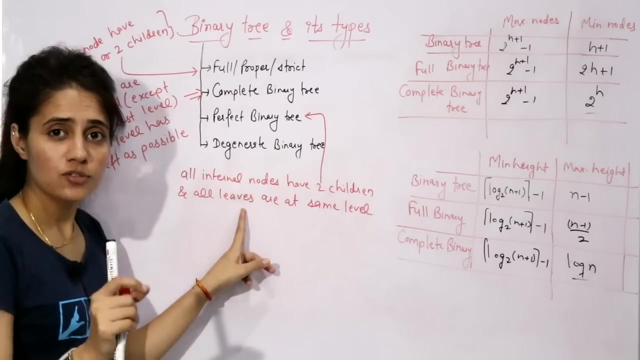 n Right. So this is what a complete binary tree, Now perfect binary tree. See, a tree can be a perfect binary tree if all the internal nodes are having 2 children and all the levels- sorry, all the leaves, all the leaf nodes are at same level. 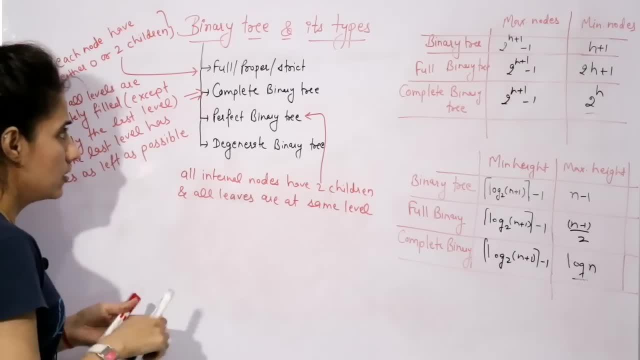 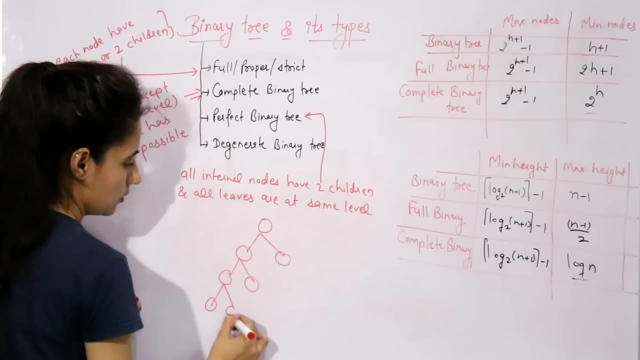 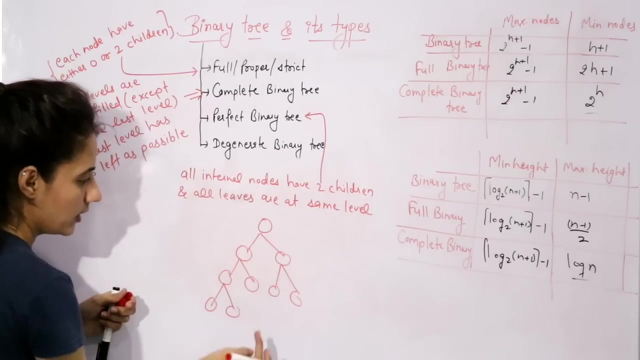 Right, These 2 conditions. Fine. Now see, I am drawing one tree. All the internal nodes should contain exactly 2 children. So here these are leaf nodes, but all the internal nodes are containing how many 2 children? 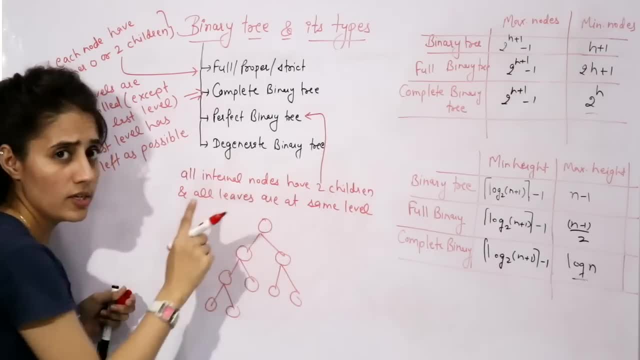 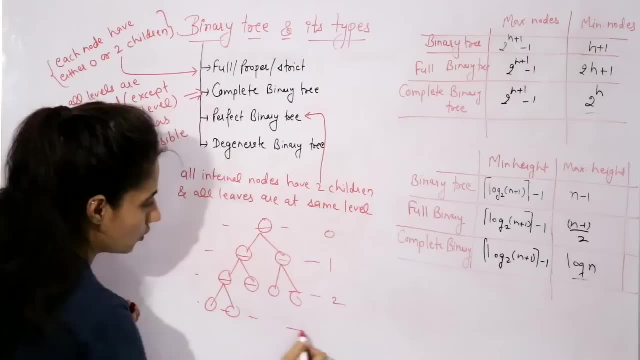 Right. But second condition is what? all the leaf node, all the leaves should be at same level. But here see, this is what level: 0,, 1,, 2 and this is what, 3.. Right, So 2 leaf node are at level 2,, 2 leaf node are at level 3.. 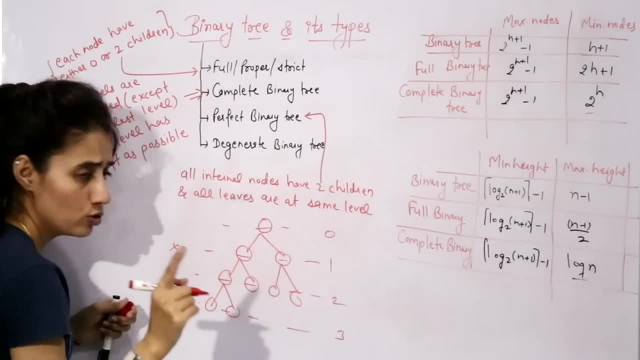 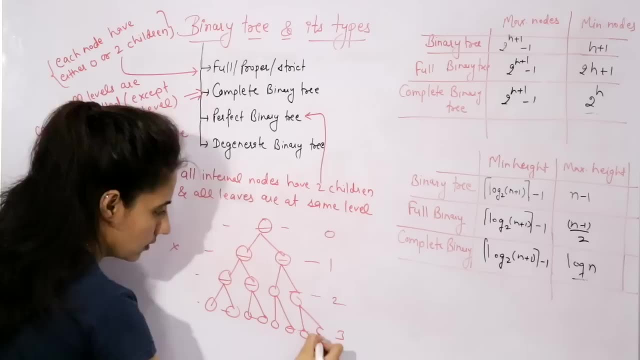 So this is not a perfect binary tree. All the leaf node should be at level 3.. So now, how to do this thing? Now see, these are leaf node and all the leaf node are at level 3, and all the internal. 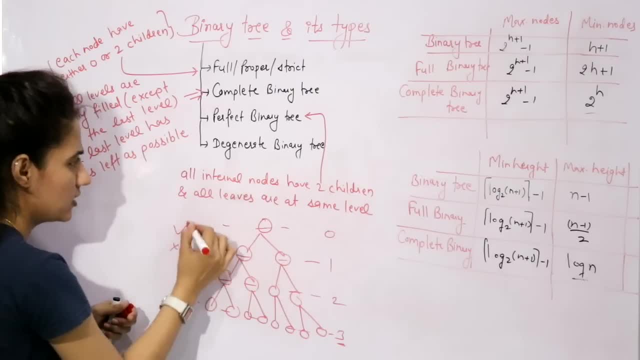 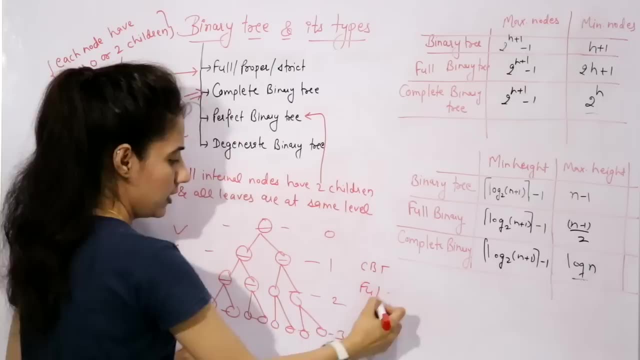 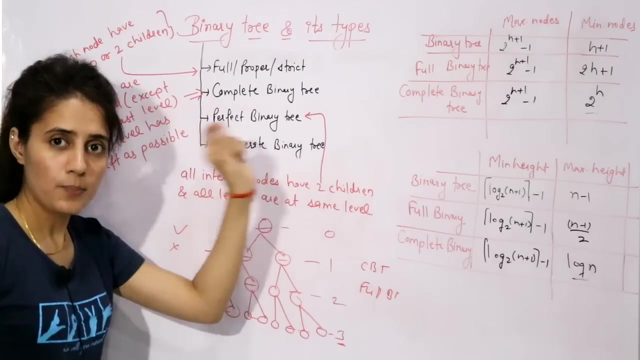 nodes are having 2 children. So this is now a perfect binary tree. Now see, this is also a complete binary tree. Can we say it is a full binary tree? Yes, it is also a full binary tree. So every perfect binary tree can be complete binary tree and full binary tree. 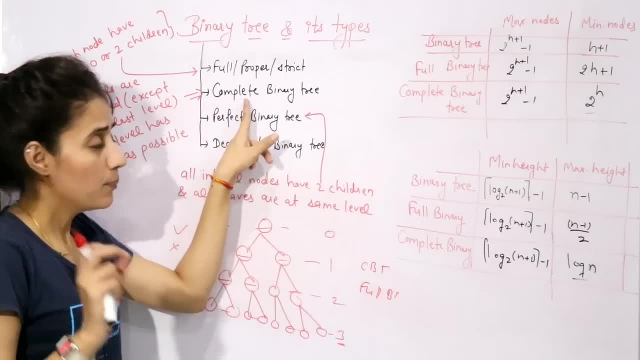 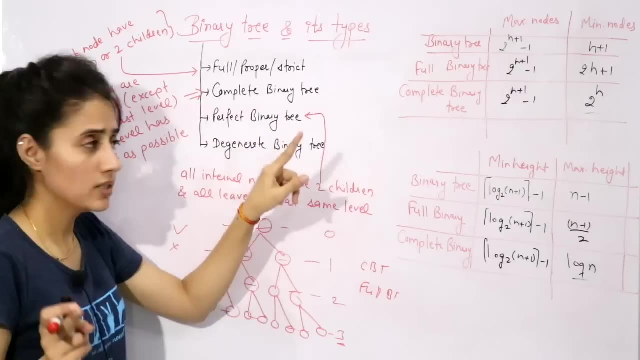 But vice versa is not true. See, if a tree is complete binary tree, then it is not necessary that it is perfect binary tree. If a tree is full binary tree, then it is not necessary that it should be perfect binary tree, Right. 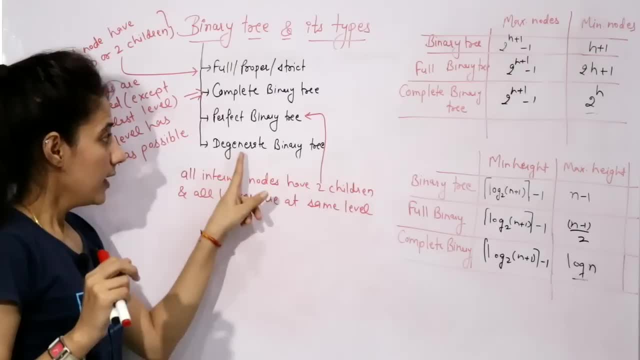 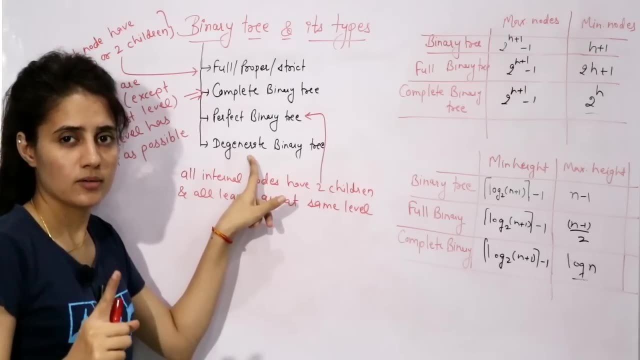 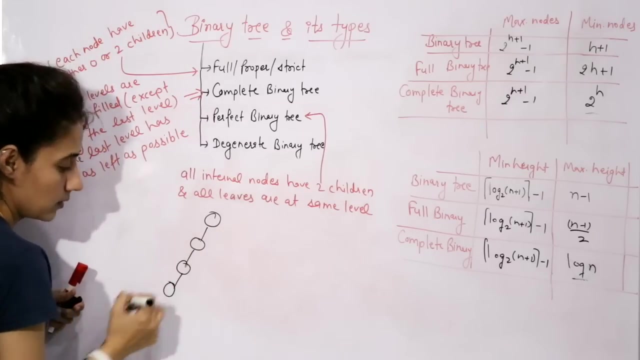 Now see what is degenerate binary tree Here. in this case, All the nodes, all the internal nodes, are having only one child. that is known as degenerate tree. So see this: If you draw this thing here, this is leaf node and 1,, 2,, 3, 3 are internal node and 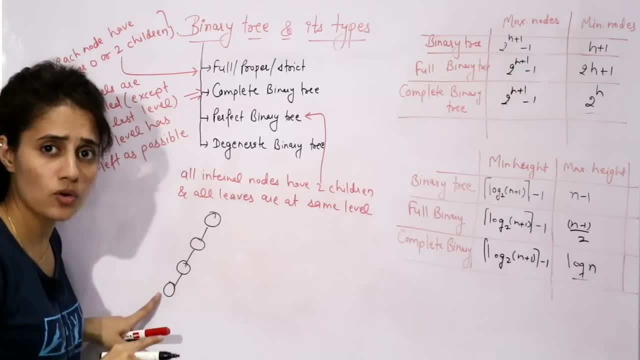 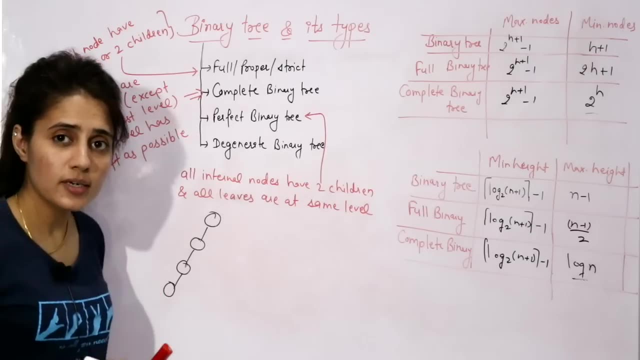 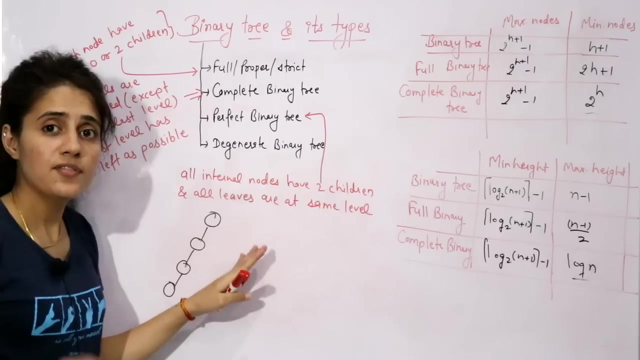 each internal node is having only one child. So this is what a degenerate tree and you can say this is what a left skewed binary tree. Left skewed binary tree means if the nodes, the internal nodes, are having only one child, then it is known as also known as left skewed binary tree. 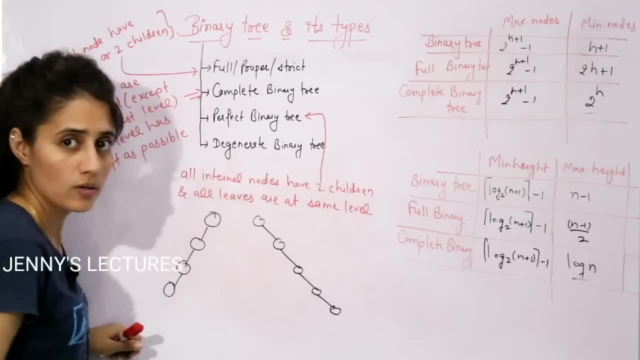 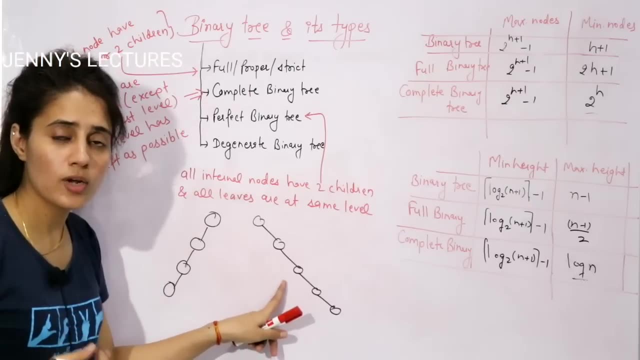 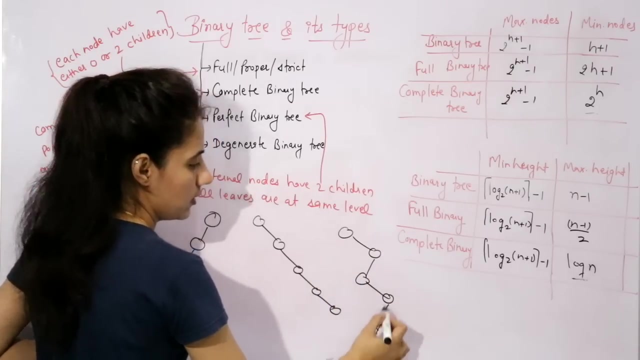 See now this tree. This is what This is also degenerate tree because each internal node is having only one child, that is right child, So it is also known as right skewed binary tree. Right Now, taking example of this, Is this a degenerate tree? 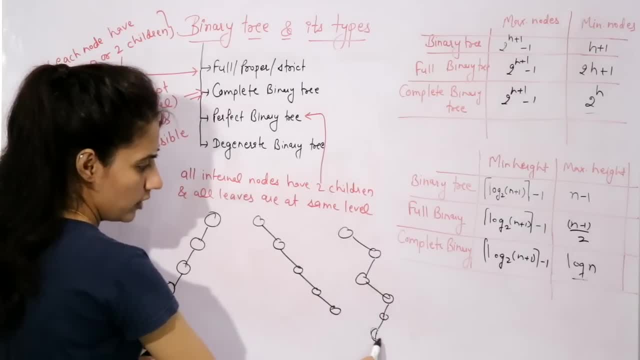 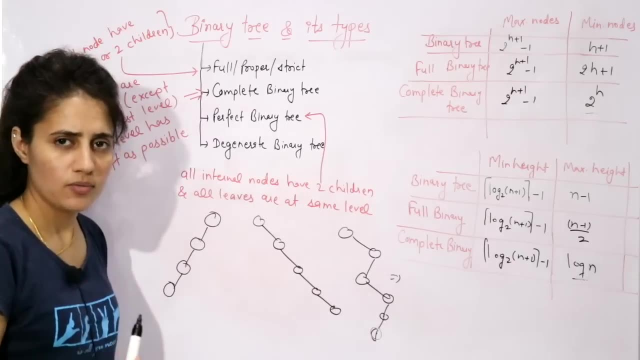 Yes, Because, see, each internal node is having only one child. One child, This is having right child, This is having left child Right. So this is also a degenerate tree. We cannot say that it is left or right skewed. 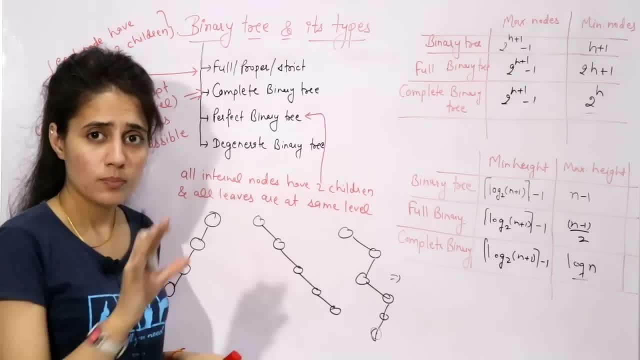 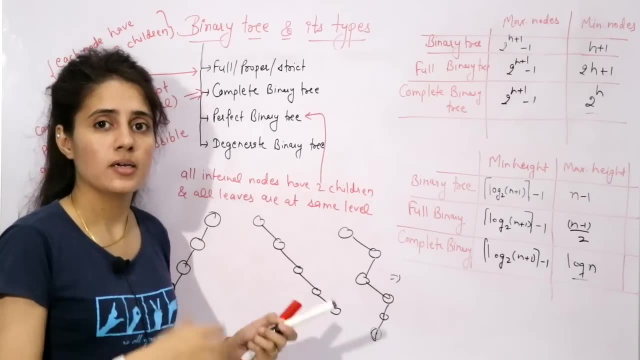 It is mixture of both, Fine. So I guess this is all about binary tree plus properties of binary tree. we have discussed and types of binary tree Right Now in detail how to implement a binary tree- that thing we are going to discuss in next. video. So I will see you in the next video. Till then, bye, bye, Take care. 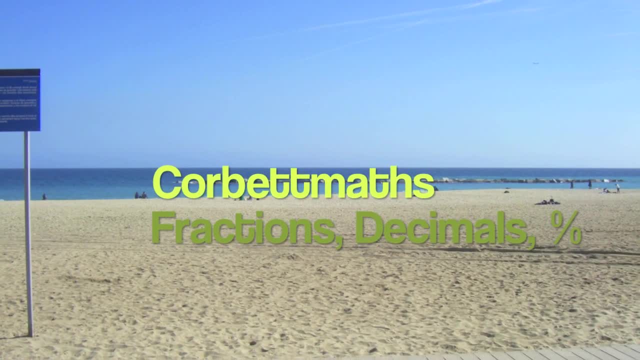 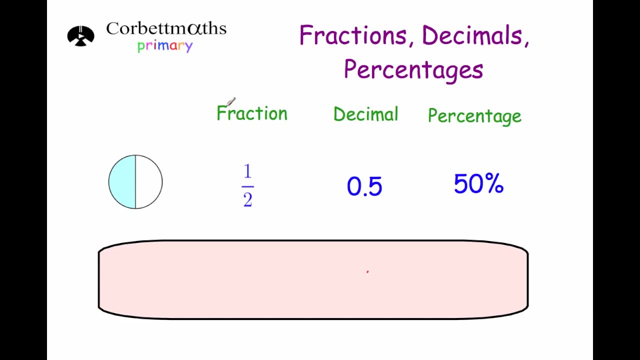 Hi and welcome to this Corbyn Maths primary video on fractions, decimals and percentages. In this video we're going to look at some of the key equivalent fractions, decimals and percentages. So here we've got a circle and half of it is shaded in blue, so that represents.